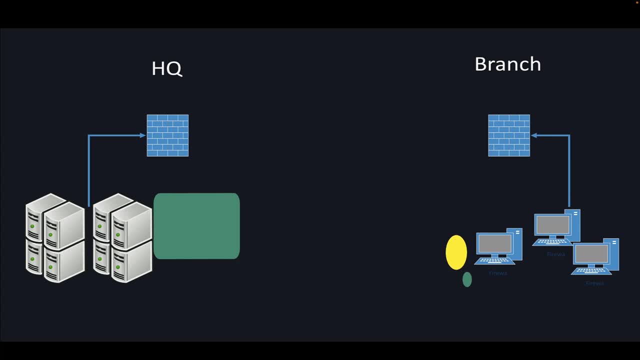 branch branch office and they are also connected to the all the all the system in the branch are connected to the firewall. Of course they are connected via the switch, but I'm just showing you the high level. and then this is the subnet for headquarter and this is the subnet for the branch. Of course there is 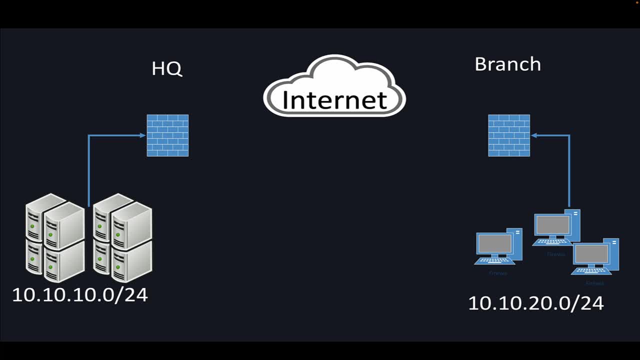 internet from where we can connect these both. There is another method, like leased line MPLS, but those options are very costly and, yeah, you need to pay more. However, internet is not that much costly. It's very cheap and with less amount of money you can get more speed. So we will. 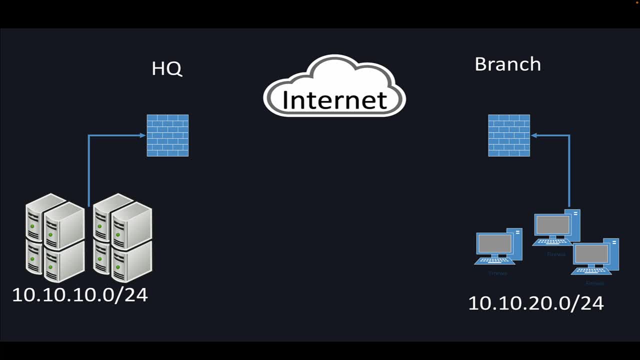 choose the internet as an option. So what we need to do to connect over internet, We know internet is not secure, so we need to configure some kind of tunnel to connect these two offices. So we will use here IPSec tunnel. Okay to connect. 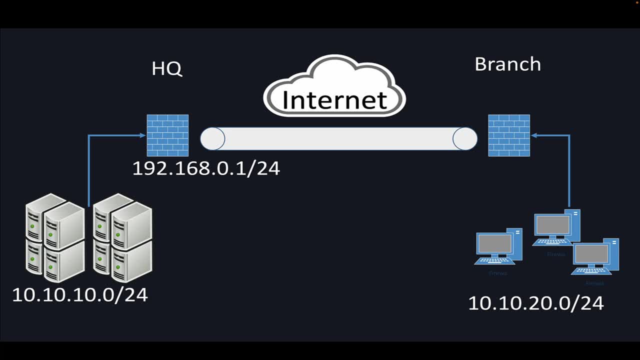 both the offices with each other. we need to have some kind of IP address in our external interface. Here I have just added the private IP address, but in your scenario it will definitely be some public IP address. So let's take these two IP address in our scenario. So this: 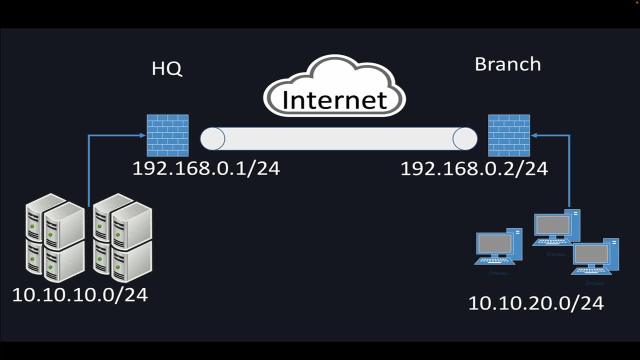 is how the connectivity will look like. So now you understand why we use the IPSec VPN to connect two different offices together and why they- why we want to connect them together. Let's take an example. in headquarter, there are so many servers which has to be accessed by the 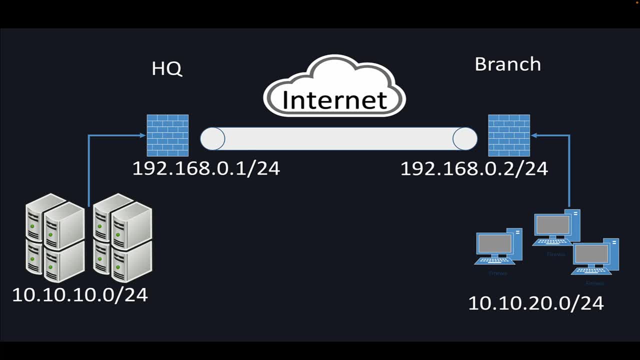 other employees, but those employees are not in the, not working in the headquarter, but they're working in other locations. You just take an example: your headquarter suppose in London and you have another branch which is in India, Mumbai. So Mumbai want to access the applications. how they will access? Okay? 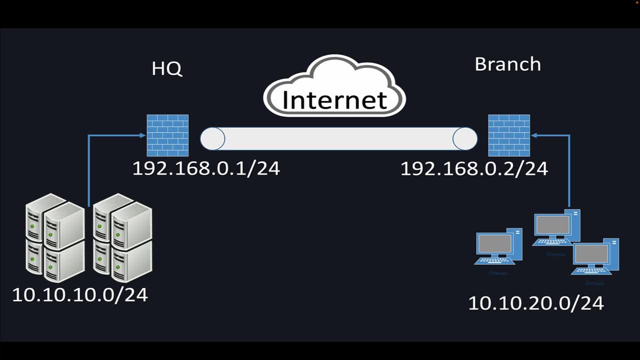 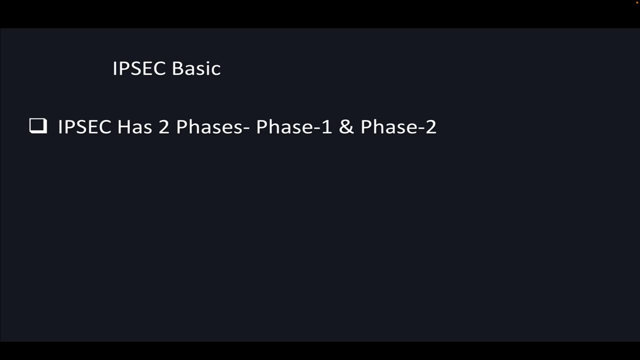 so they cannot go to headquarter, but of course, they want to access when they're in Mumbai. That's why we create the VPN. Okay, so that's the purpose of creating the IPSec VPN. Let's go to the next IPSec VPN basics. How many things you need to know as part of the 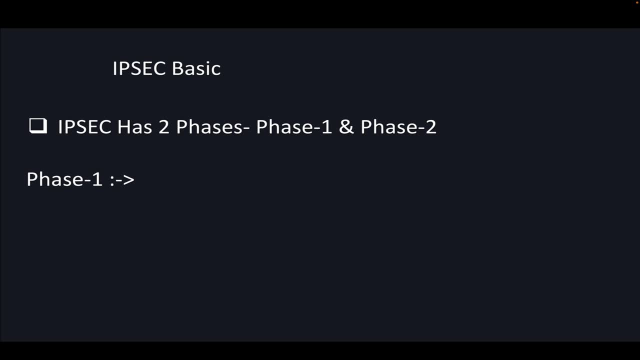 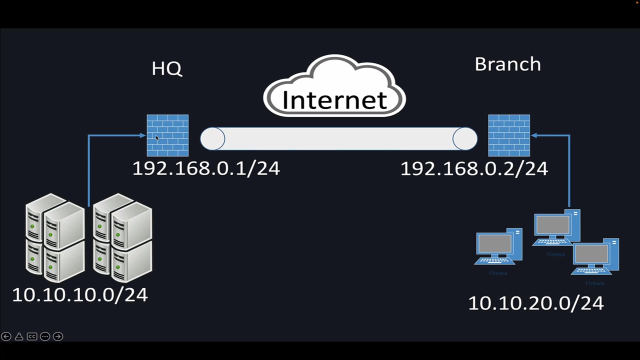 IPSec VPN. It has two phases, Phase one and phase two. Phase one is used for the device negotiation. It exchange couple of messages. Device negotiation is like. if we go back to our previous diagram we know that if VPN has to establish, it has. 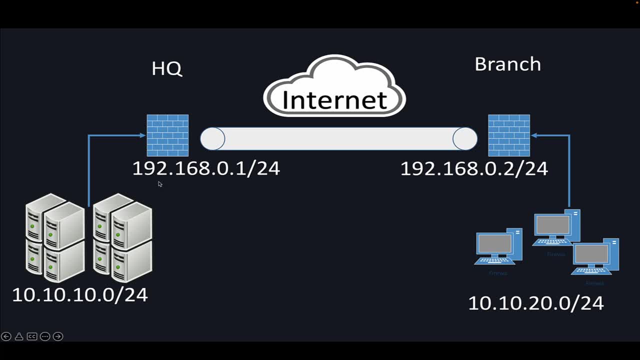 to establish between this and this firewall. Of course, once the VPN is established, the data will start transferring. Okay, suppose here there is a payroll website in our headquarter and these guys want to access this website over the VPN, right? So after establishing VPN, this traffic will go. But before that. 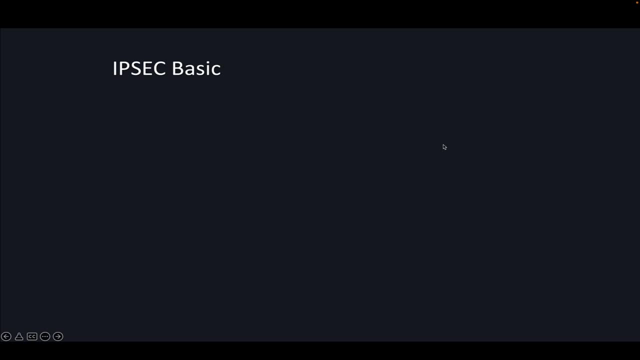 these devices need to negotiate, They need to create a VPN, and that's the way to do it: Phase one In phase one, device negotiation happens. They exchange a couple of messages. So now you might be thinking how many messages they negotiate and what are the different? 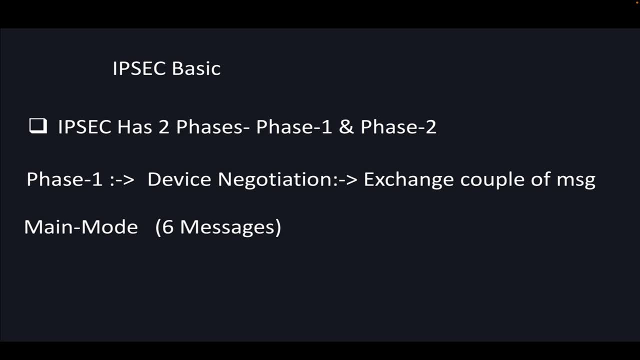 ways to exchange those messages. So there are generally two modes in phase one. One is main mode, which has six messages, and another mode is aggressive mode, which has three messages. Keep in mind that these messages are exchanged between those firewalls. So if you want to, 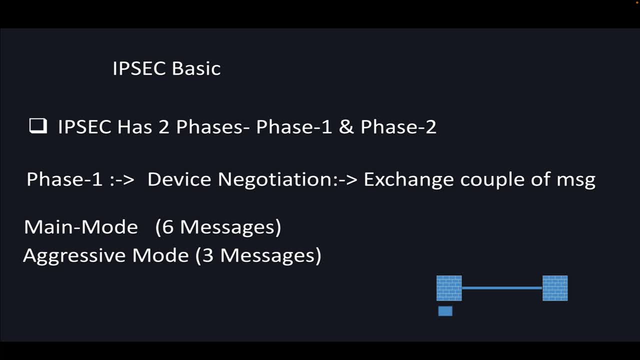 have two firewalls, as it is mentioned. it happens The negotiation happened between the devices, Device negotiation. Okay, so these two will negotiate the message, They will agree on them and then phase one will become up. Okay, so we know now phase one and there. 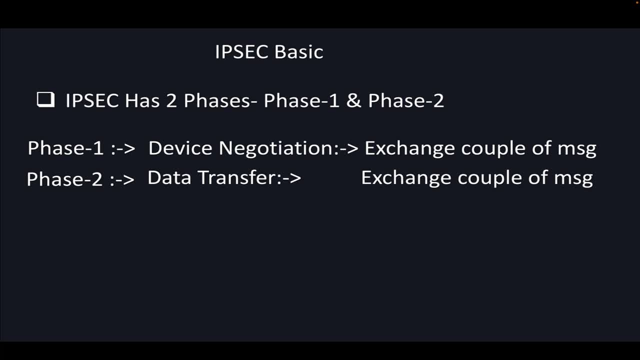 is a phase two and the purpose of phase two is the transfer, the data. Okay, for transferring the data, the good thing is there is a phase two and there are also a couple of messages has to be exchanged, so that phase two tunnel will become up, So you can also. 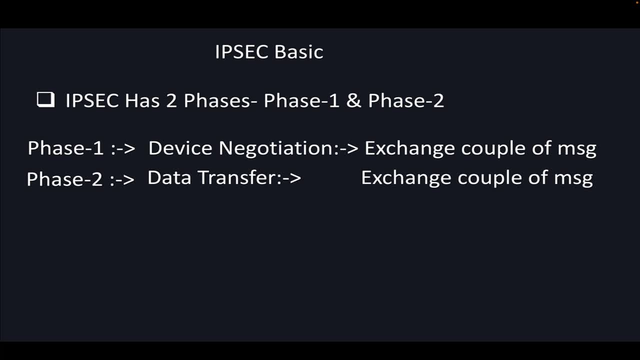 consider phase two like a tunnel inside tunnel. Phase two goes inside of phase one, so it's more secure, Right? So now again the same question: How many messages are being exchanged? So there are three messages being exchanged, and in phase two we only have one mode. that 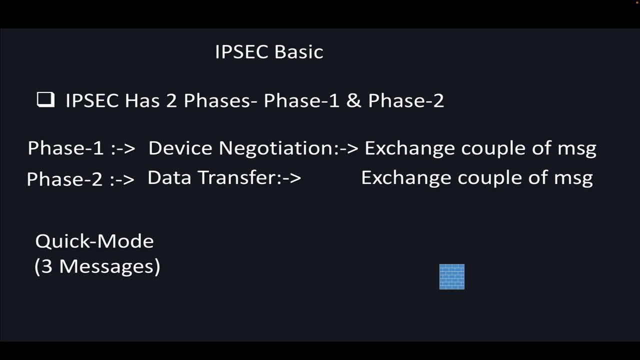 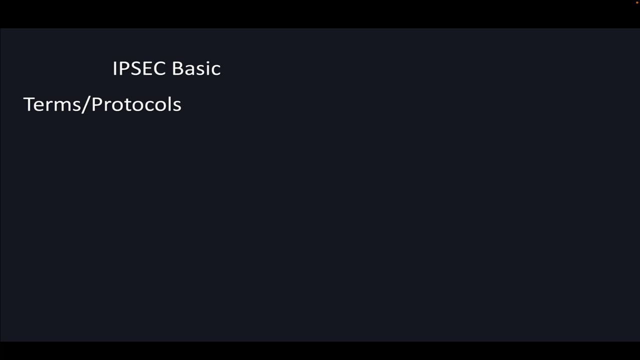 is quick mode. Okay, so this is the high level of IPsec VPN. Again, the same thing. Once the negotiation happened. phase one is up, phase two is up. then the data transfer will take place. Okay, so these guys will start accessing the application. Okay Again, continuing on. 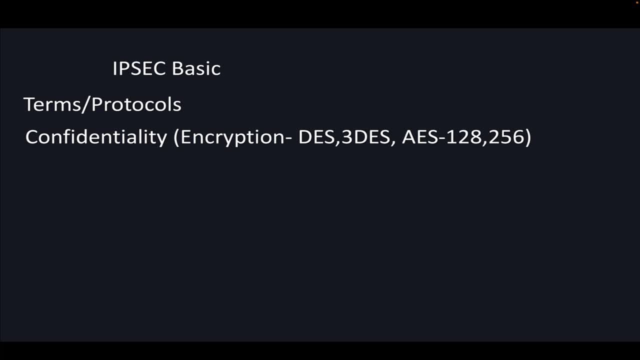 the IPsec basics. There are other things that you need to know Why we use IPsec. you know like to connect two devices, to connect two offices together so they can access the things like branch office can access the applications placed in the headquarter. 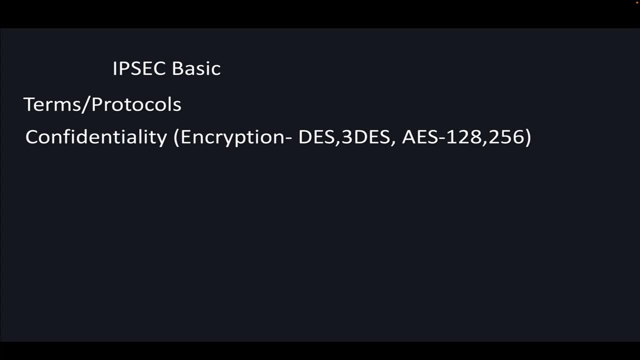 Like for the sake of the security. there are three things that you need to keep in your mind with IPsec, which is confidentiality, integrity and authentication. If you see the confidentiality means your data is confidential. Nobody else can see your data And how it happens it happens. 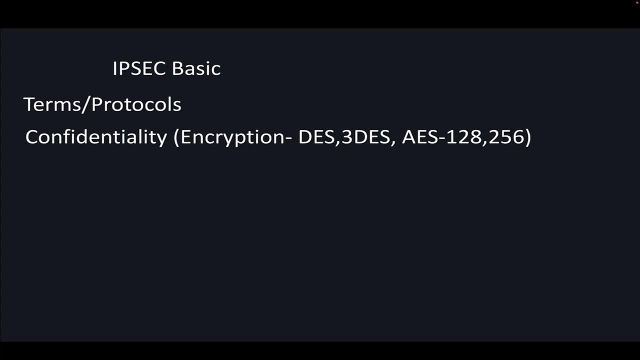 with the help of encryption And there are different methods for encryption: desk, three desk. they are really weak, but you will still see the options. a couple of devices, However. they are strong methods, which are which are AES 128 and 256.. You can use 128, that is. 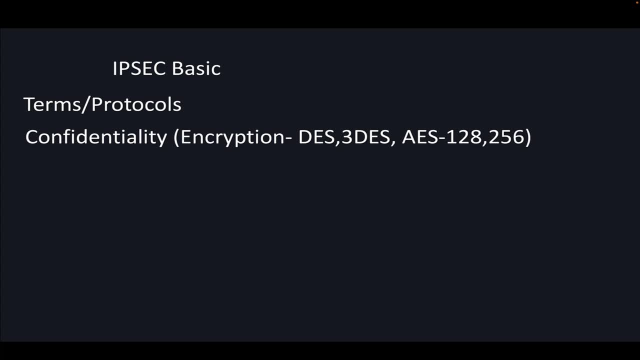 also secure. 256 is way more secure. But please keep in mind that if you will use higher algorithm- like instead of AES 128 you will use AES 256- your file will need to do more processing to encrypt and decrypt the data. It could spike your CPU and RAM If you have a computer. 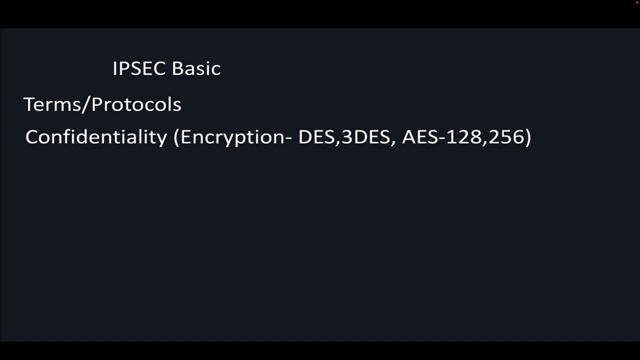 with a good firewall with very good configuration, like high CPU, high RAM, big model, you don't really need to worry about that. you can just go ahead and use 256.. The next is integrity. integrity is like hash. you can say hashing. We use integrity. that for the reason that. 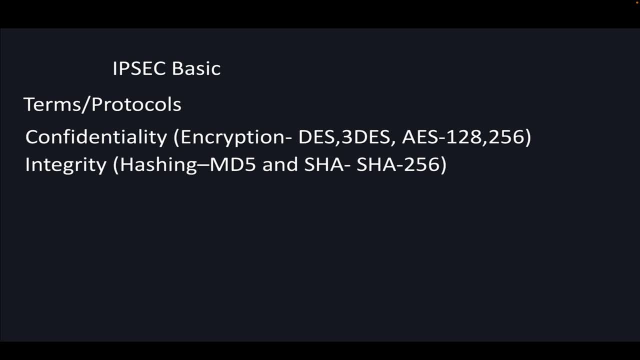 your data is going from one place to another place, It should not get changed. like you sent some somebody hundred dollar, They should not get changed to ten Right. This is just an example. With the help of hashing we achieve that integrity that is not changed. There are different algorithms for that: MD5 and SHA. MD5 is a weak and there 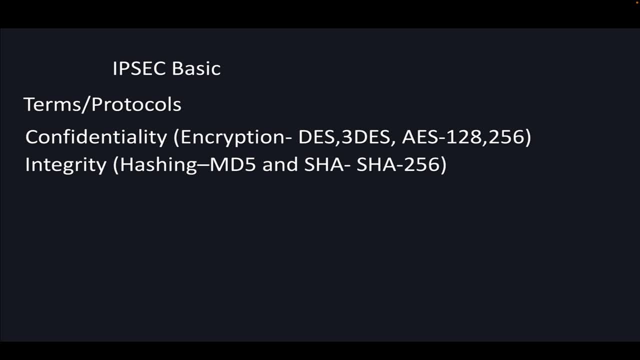 are many versions of MD5, but all of them are considered weak, So better use SHA, SHA. again, SHA 256 is the strongest. you can use, that, OK. And the third thing is authentication. For authentication, we have two choices again: Pre-shared key and separate key, So you can. 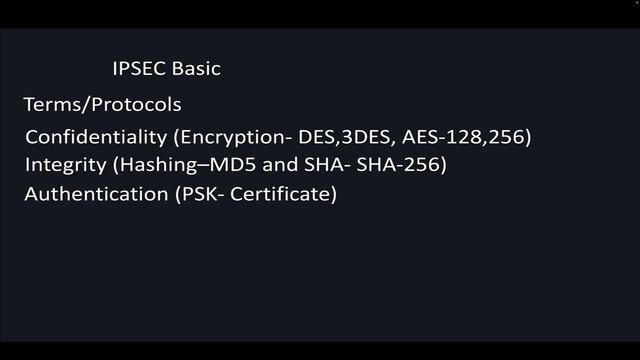 use one of your three or more certificates. Most of the cases you will see everybody is using pre-shared key. OK, But the best and the secure method is to use these certificates. OK, so there is another thing that you need to know: HADL- that's a short form- created. 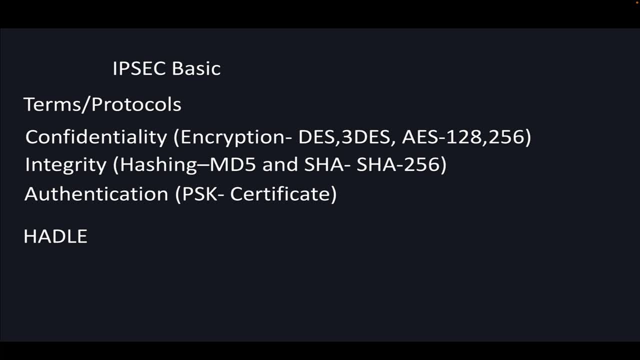 by somebody, not by me, And this is a really nice short form to remember the couple of messages being exchanged. If you remember, I have told you that in phase one there is a main mode and aggressive mode. in main mode, six messages gets exchanged. now this is time to think what goes. 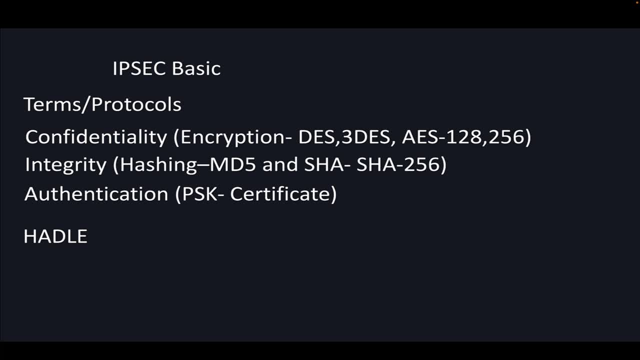 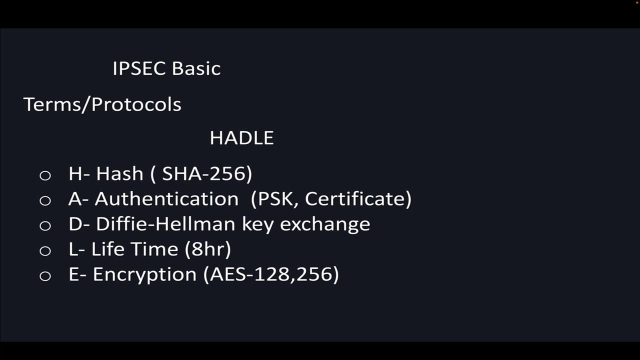 inside those messages. okay, so handle is the information which goes through those messages. h is hash, a is authentication, d is diffie helman, and i think- yeah, i think here i have mentioned it completely- uh, h is hash and in hash. again, we just discussed sha-256. let's take an example. we are 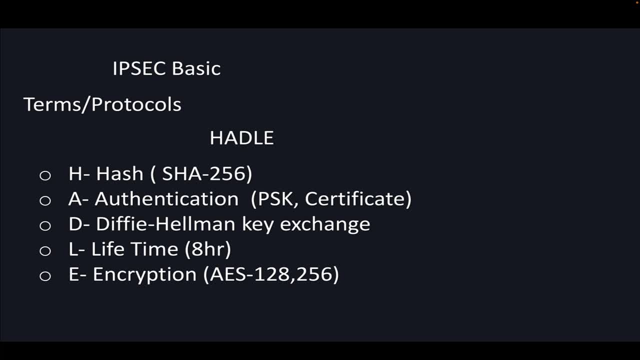 using sha-256 and then authentication. you have two options: appreciate key and certificate. diffie helman is a key exchange method. this is a different topic. you can go ahead and check and do search on that. but db helman, um, with the help of diffie helman, we create a shared secret key, okay, so? 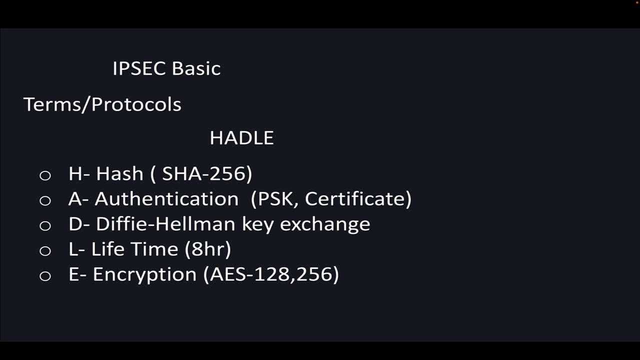 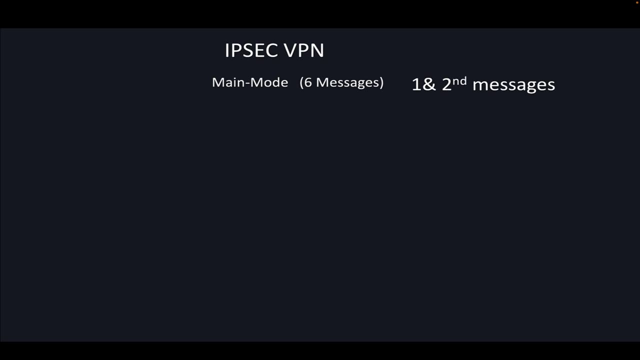 uh. another one is l, that's lifetime. just take an example that your key will not be expired, uh, for eight hours. okay, that's why we use lifetime. then we use encryption. uh. for encryption, you can use aes 120, error 256. okay, now let's see: uh, what are the messages? uh goes inside, so there. 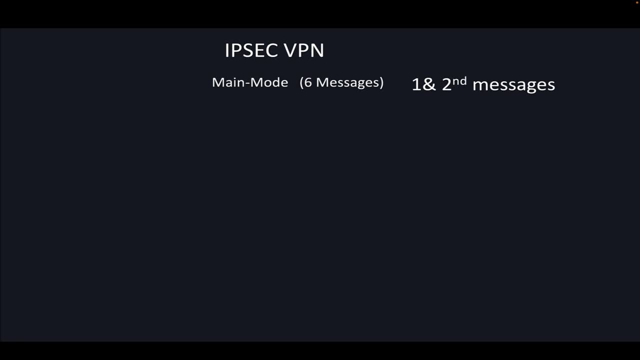 are, of course, six messages, but the good thing is like you don't need to remember all the six. first message and second message are same. the only difference is the first message is being sent by initiator and the second message is just responded by the responder, so we have two things here to notice. 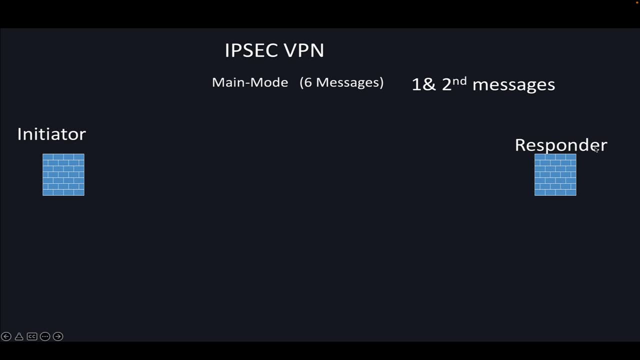 initiator, who will initiate the communication? responder, who will respond to the communication? okay, so, as i explained to you in the previous slide, handle information will go right. so initiator will send the handle information and responder will send its own handle information and then they will say all okay, and let's go to the. uh, let's go and send the third packet, which is: 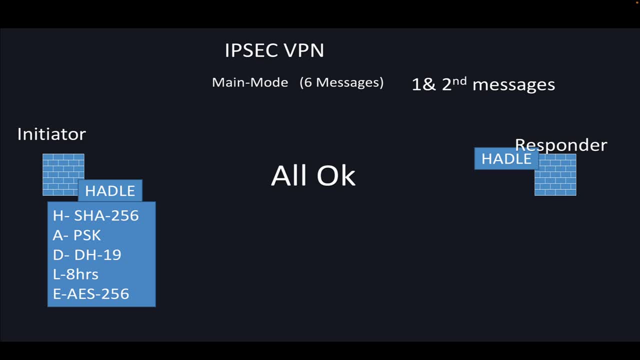 i will discuss in a couple of seconds. uh, before going to the third packet, let's see what goes inside. that we just discussed handle. this is the information that they share with each other. they just uh. another thing to notice. they of course say, okay, let's uh use sha256 for. 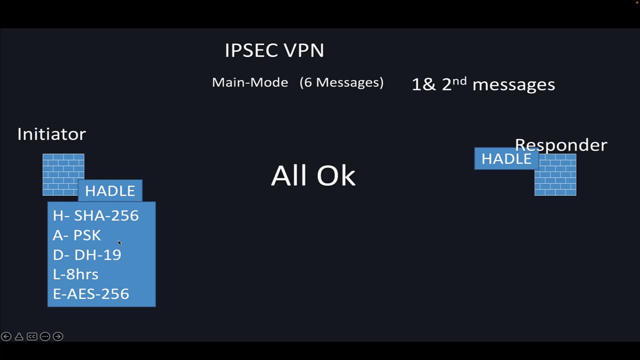 authentication. i'm not going to use digital certificate. i will use pre-shared key, but i'm going to use the shard256 as a hash. and also another thing to notice, for an example: for question perspective or exam perspective: if somebody is asking you like your password goes, 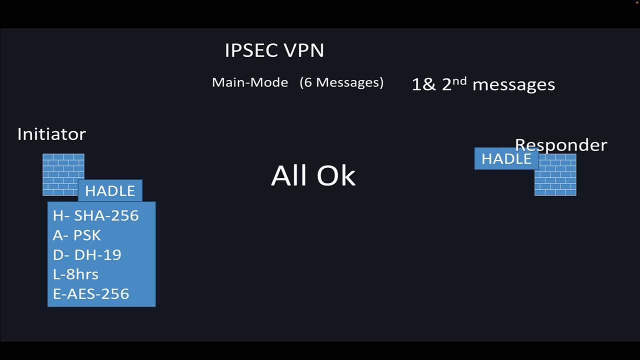 inside a first message. no, password doesn't go in first message. first message is all about, uh, the methods that we are going to use. okay, so we are going to use the sha256 as a hash, but hash doesn't go in first message, only the method goes in, that algorithm goes in that and. 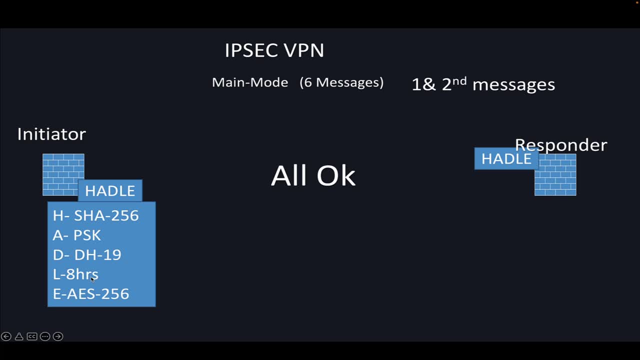 we are going to be using shard256 as a hash, and so we have different ways to use sha256. so let's go to alert mode and we'll uh activate the alert mode. that is the remaining one. we'll go to an alert mode and turn on the alert mode. see, the alert mode is active. 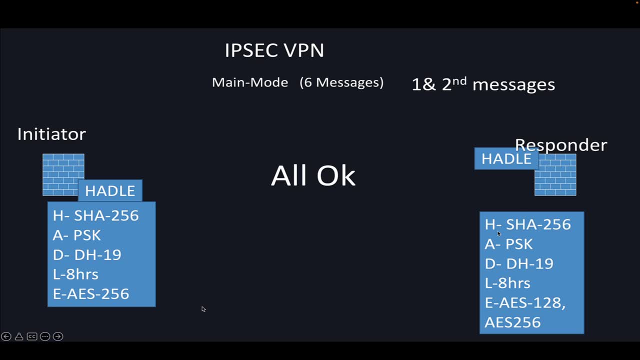 when we activate the alert mode. it allows us to do a based on our timetable. so the alert mode will turn on automatically as the alarm went off, which works in a simple way. if we have an alarm mode, for example, suppose we are using 19, suppose a lifetime, we said okay, 8 hours. and encryption, we are using 256, another guy will also reply with that notice here. another thing: so all other things i have kept same, but encryption. you can see, i just mentioned a s128 and 256. the responder or another party can have more than one encryption or hashing, ok, but he should have at least the one. 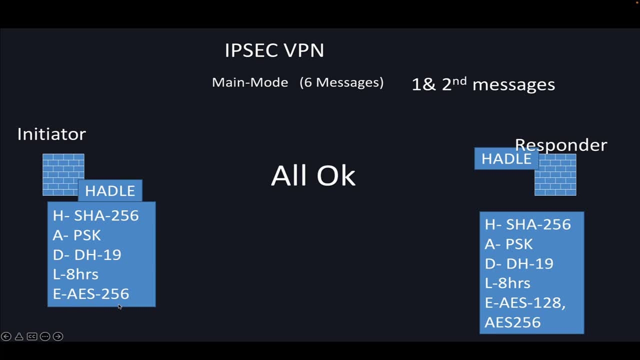 with matching with another party. okay, why that? so it's exactly same, as suppose you are going to talk with a person and you know english, then another guy knows chinese, but if he also knows english, then you both can talk with each other. but he, if he doesn't know, uh, english, but he know. 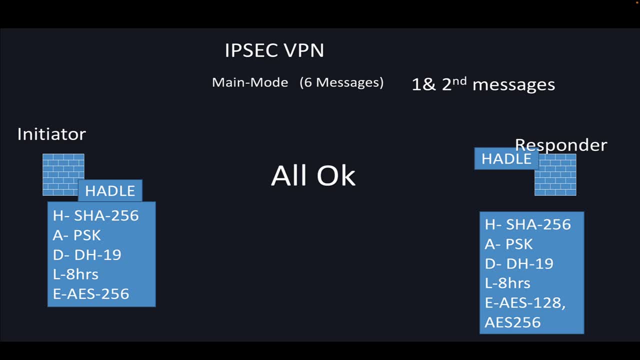 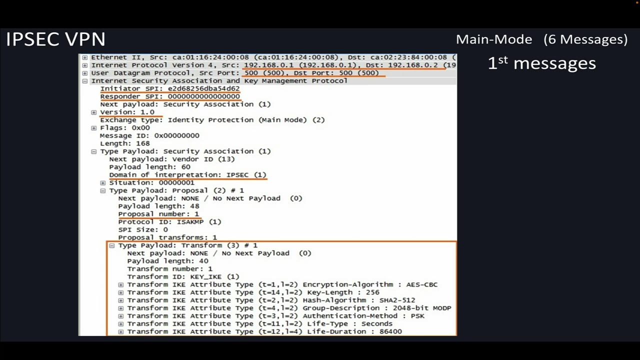 chinese, you know spanish, so many other languages, but he doesn't know english, so you cannot talk to him, even though he has so many- uh, knowledge of different languages. okay, that's why at least one should match. you can have more than one, okay. so now it's the time to go a little bit. 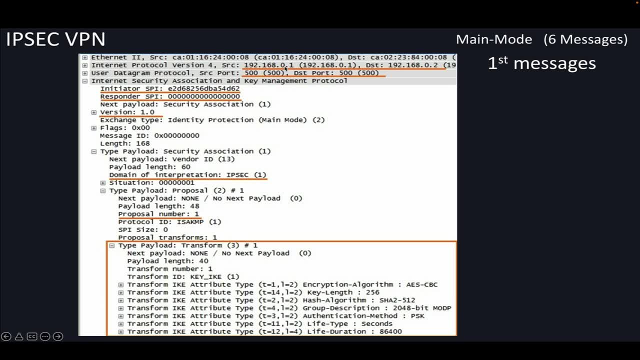 interesting see, interesting picture. so the first message, it is, of course, from the initiator which we have seen here. initiator, he will send the message. if you remember, we have this ip address: 0.1 and 0.2. 0.1. 0.1 is: 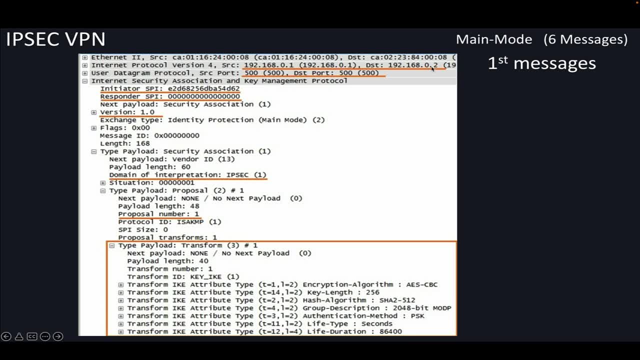 0.1 is our initiator, which is source, and 0.2 is our responder. that will become the destination. okay, the source port is 500, so 500 port is being used for ipsec vpn. we will discuss this later- and then you have here initiator and responder. okay, so there is a initiator value that's called 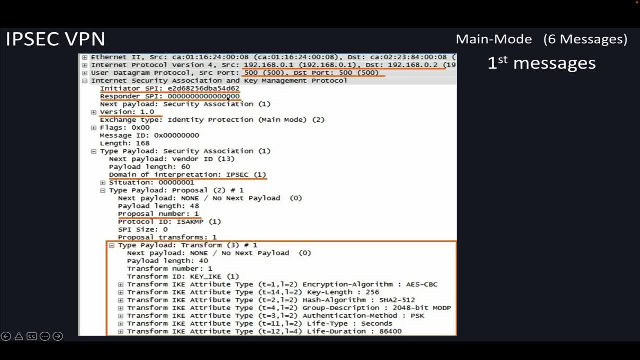 spi: initiator value and responder spi. responder spi is always zero. this is how you identify the message. second message will be exactly same, but how you will identify if it is first message or second message. this is from here. you will identify responder spi. okay, and then we are: which version? 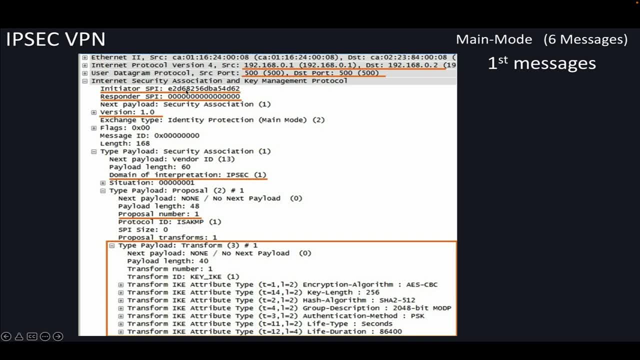 we are using. we have isa, kmp internet security association key management protocol. there's something else you need to remember. this is used to share this. this is complete protocol used for key management protocol. so this is used to share this. this is complete protocol used for key management protocol. 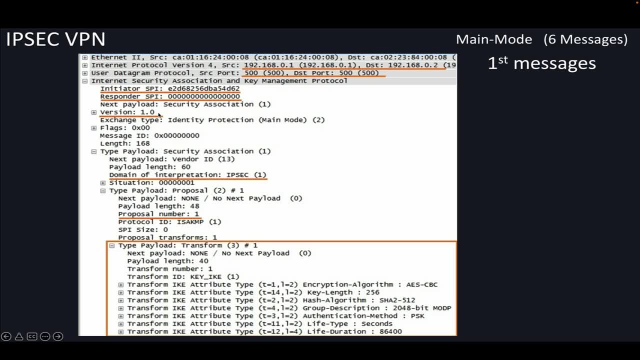 okay, so we have 1.0 version that we are using inside that we can use ike version 1 and ike version 2, but i have not explained you that, so you can just avoid that and then you can see: this is proposal number one, that's. this is here the interesting part comes. i've told you that in first message. 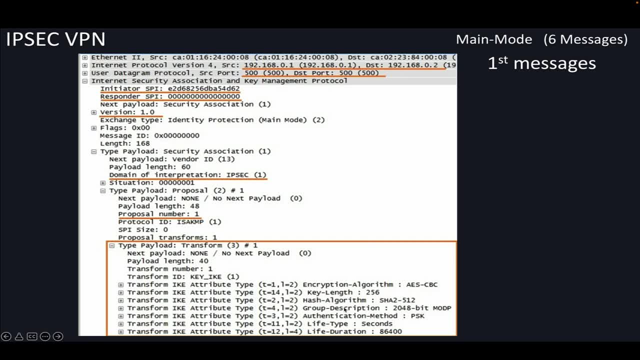 hedl information goes, so hedl can be up and down. okay, so that's just for you to remember. so in hedl there was e. that's in hedl. there was e that's in encryption. so you can see a, b, a, e, s, c, b c. the key length is 256 for 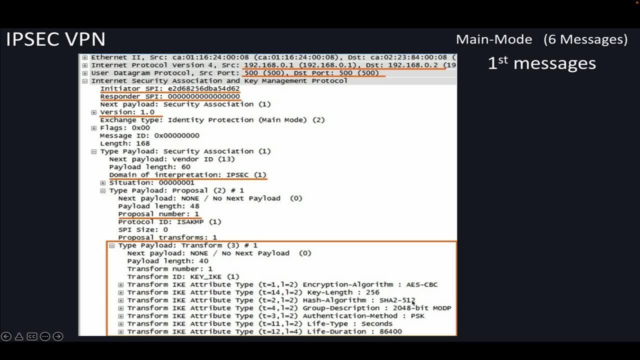 encryption uh hash algorithm. they are using sha 2 512. that's really strong uh group description. is this one 2048? by the way? i have taken this from the internet. uh, this screenshot to explain you. i think it's interesting for you to understand how it looks like in a white shark. 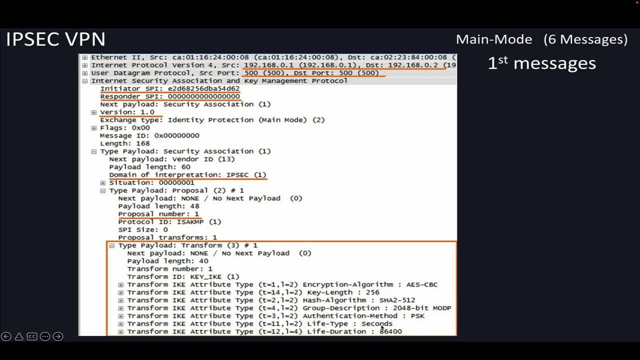 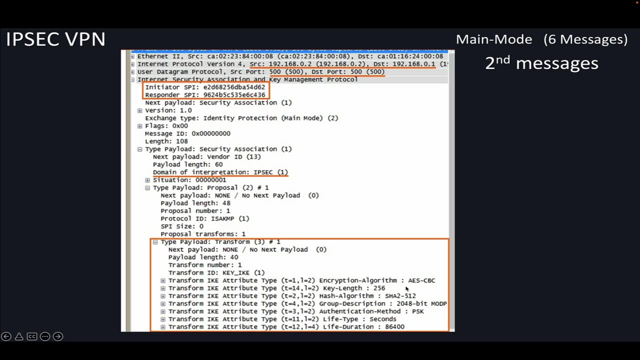 so authentication method, we are using preset key and am Alternative giving you: đây was ہم. The second message looks exactly the same. see, everything is the same. it should match with the first message. of course, everything is the same. you can pause the video. 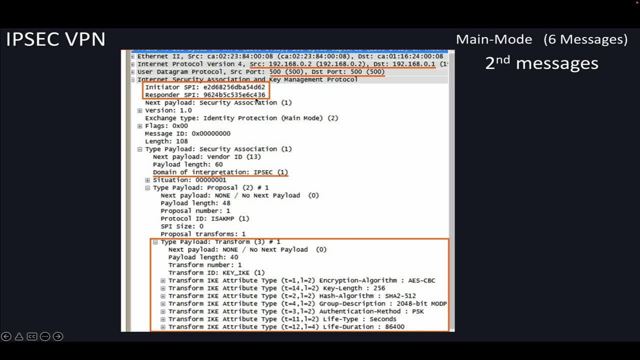 it is the same, but the interesting thing here is you can see Their起來, then you canları about the first m, not to talk about the second message. but we have the first message. Michael, let's say that we've had this request and originally when i came here it was before i. empty session guide. 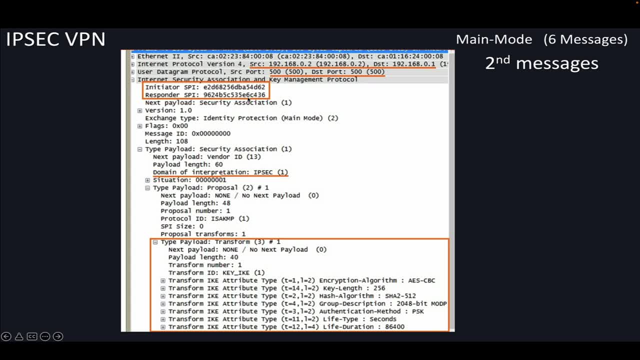 00. responder. second message will be having responder but all other messages will also be having same initiated and responder key. so the second second thing to identify second message is you need to look into this information. they are called transform, so we said handle as a short form. 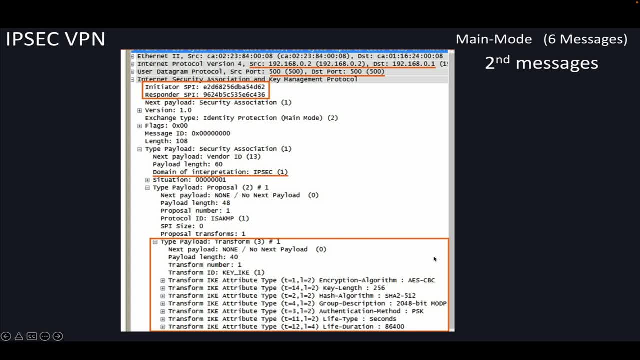 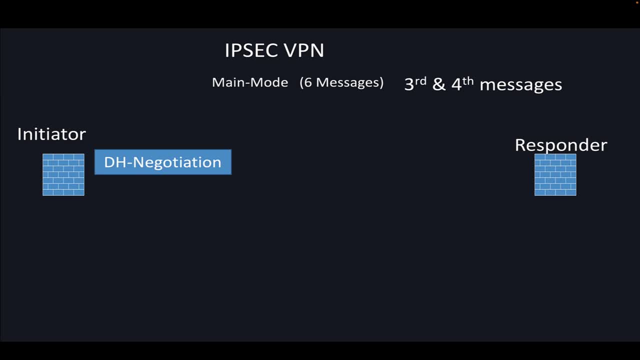 they are called a transform. this is the information they are going to send each other. okay, now, third and fourth message again. so this is a negotiation of Diffie-Hellman. okay, Diffie-Hellman. there is a group where we said, like we are using 19 group, they negotiate with each other. they could. 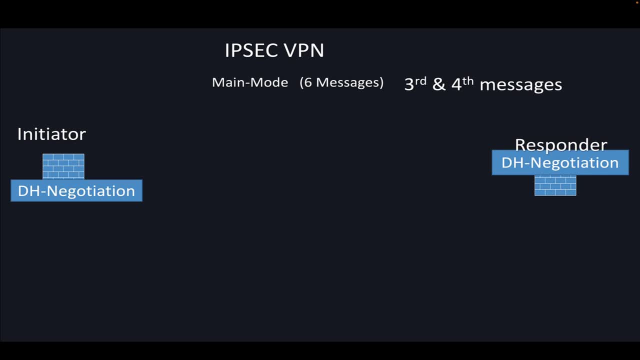 send a couple of messages, that's. there is a mathematical formula behind that and if you know about that, then you, you know how they, how it works. with this help, with the help of Diffie-Hellman, we negotiate shared secret key, okay, and if everything is okay most of the time, for the troubleshooting also, you will never see. 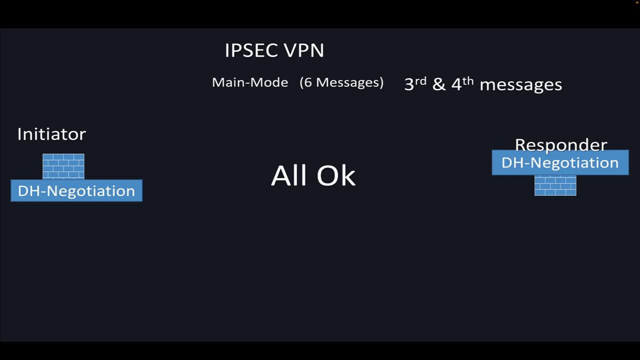 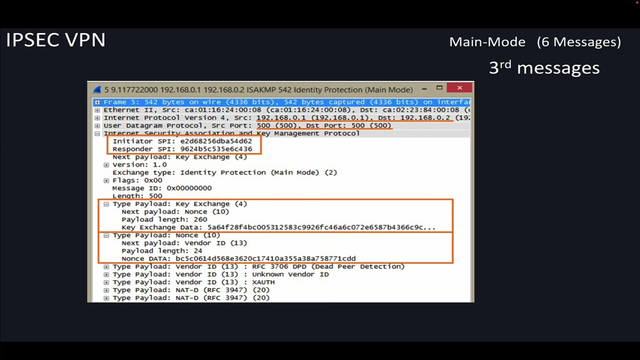 any issue in message three and four if you, if you will get a second message, you will always get third and fourth message and the problem will come in the fifth message. that's a good from into point of view and also troubleshooting point of view, how our third message looks like. 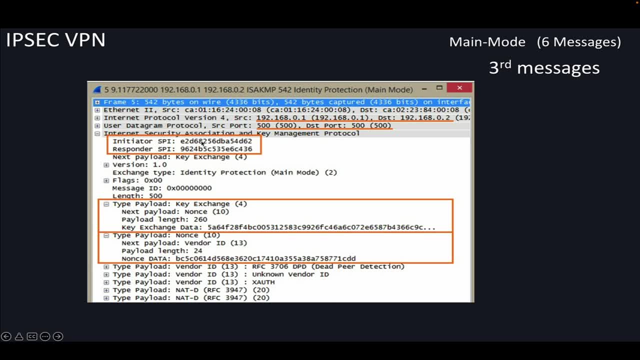 this is what i told you. if you remember, except message one, all other messages will be having same initiator and as responder spi. okay, so from here you can only identify first message if it is zero zero. you cannot identify remaining messages by looking just the packet. i can identify, uh, by just looking into output. 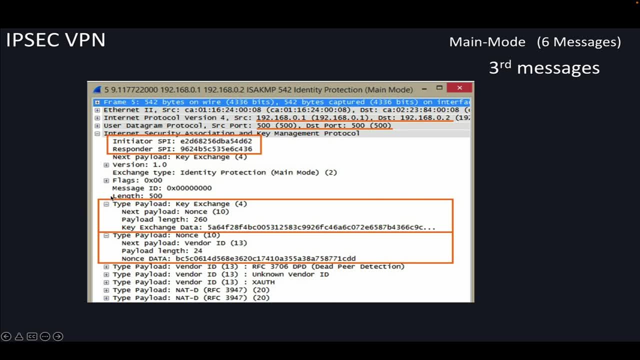 any message. if it is third or fourth, you can also do that. and how? how's that? the thing that you need to notice. in the third message, the nonce value goes: okay, this is nonce data. this is like a random value they exchange. okay, if you will know the Diffie-Hellman algorithm, you will come to know why they are. 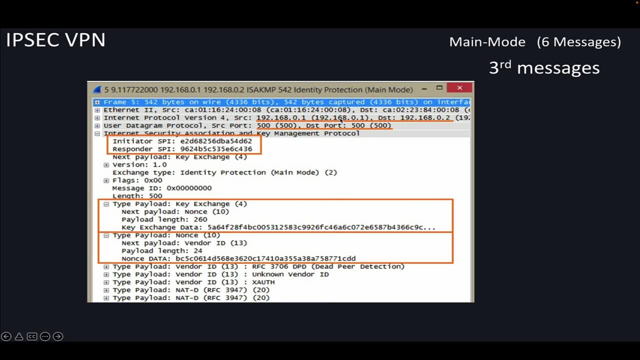 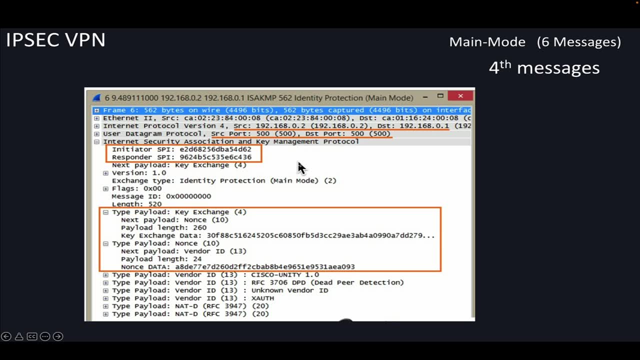 using this random value, okay. another thing is, if it is third or fourth, because that again looks exactly same. you will see exactly same. it looks like. okay, maybe the nonce is different. you can see nonce is different, but that will not make you any hint if it is third or fourth message. 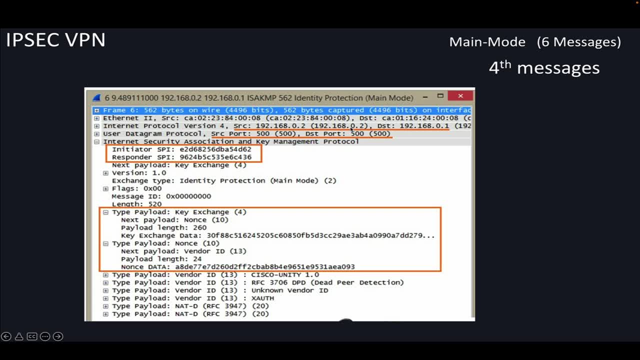 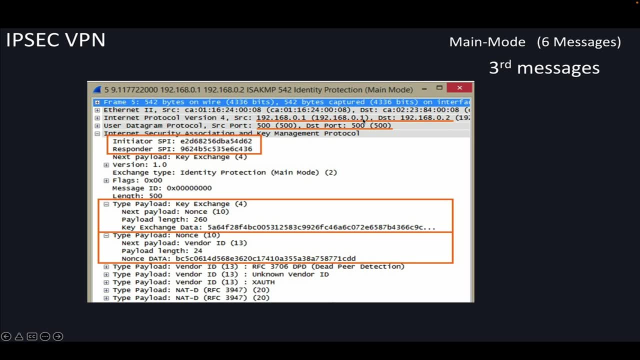 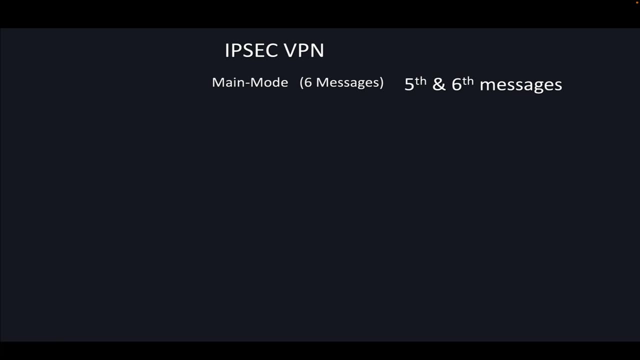 how you will come to know about third and fourth is from here: source address and destination address. if it is a, let me go back. if it is 0.1, we know this is our source and this is our destination. if it is, reply is coming. we know it's a fourth message. now let's go to fifth and sixth message. 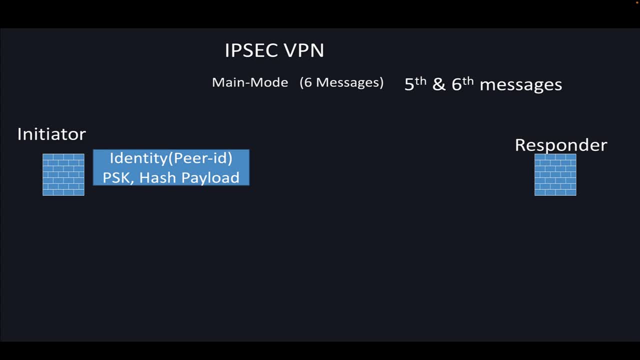 so in fifth and sixth message identity, that is peer id. when you will configure the vpn there is option as a peer id. if you do not configure peer id then ip address will go in that as a peer identity. then there is a pre-shared key in the first message we, if you remember, we have 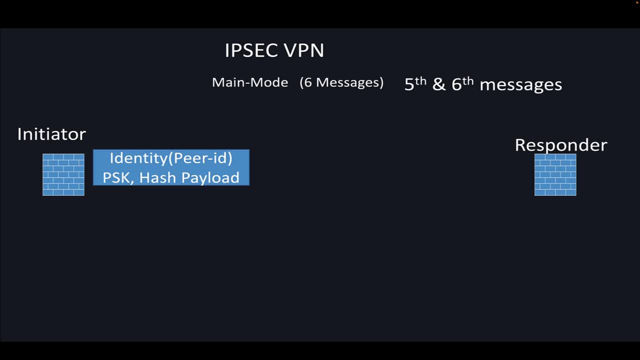 used method for authentication as pre-shared key instead of digital certificate. but the value will not go in a first message. value will go in the fifth message. what else will go in this hash payload? if you remember, we use the hashing algorithm, i think sha256. we mentioned the value. 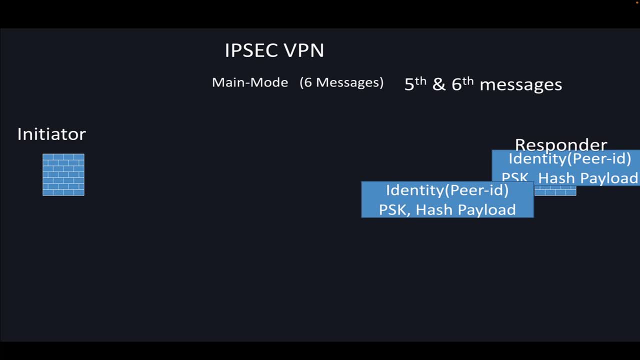 of hash atSirio, and as this is going to include not a database but a garage building part, so there are some value, values which we can target here and i will go on a key page here and we can see everybody and we can start Crystal data. ok, we have sign pages. yes, first and then leave. 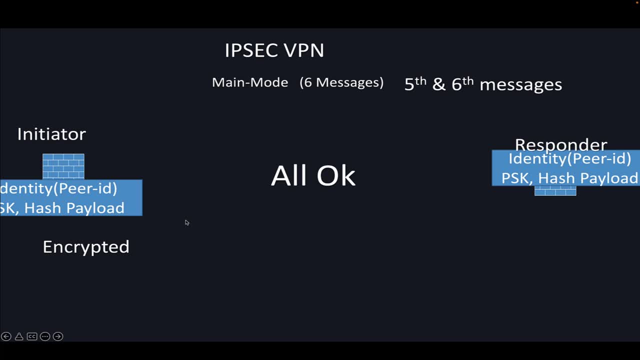 2% seed memory and finally we have hereЕТ money: 1% judgment. ok, so that means give us our� login the minimum from word refresh option. can you please let me come up here for the arrow Alt, I'm writing my name from here. now we are coming here. 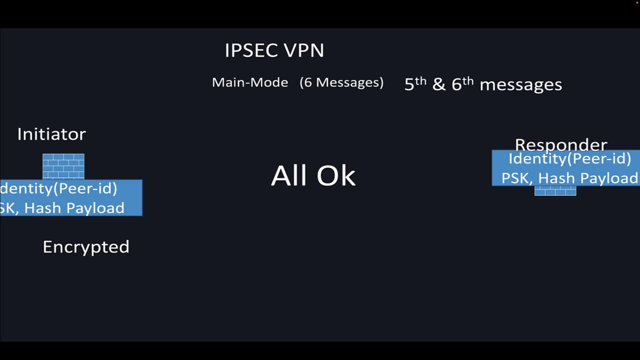 So yeah, just go into p6 default password, then goto to this message here, okay, and you can see this message is coming in and the email is coming. you can see that this message is coming just from an tech server. so, anyway, something else. what are you going to see in Islamic security window? 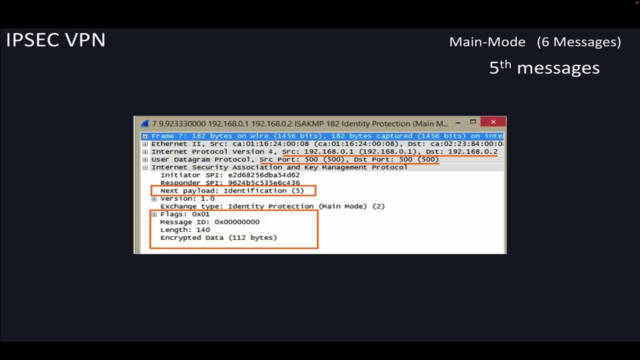 a message instead of the article. i'm going to attackpress money. he will take his作 race on the now from here. you know that fifth and sixth are encrypted. this is how it looks like they are encrypted, because pass, your pre shared key, is going right, so 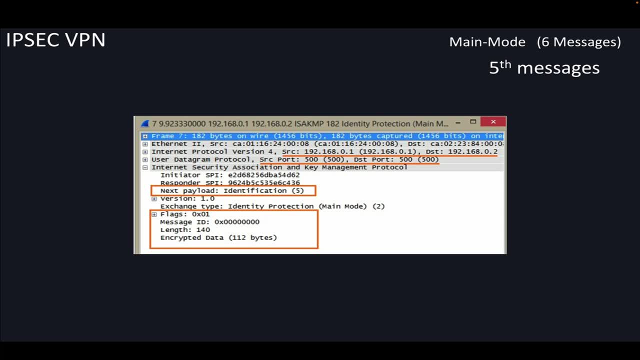 you cannot send your pre shared key- means your password- over unencrypted channel, right? so that's why they are encrypted. now, here you can see how they look like again. 0.1 is our source and this is our destination, port number 500. this is from where you can identify this identification. okay, and you will see. 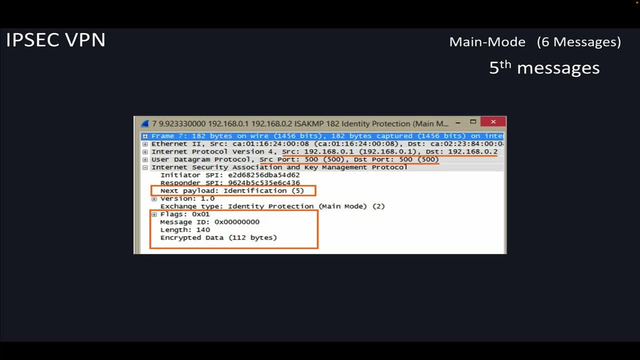 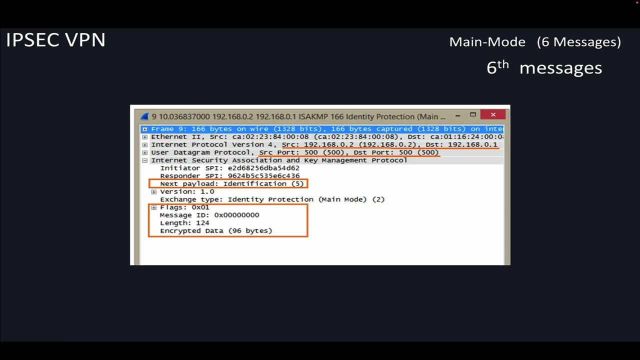 like fifth and sixth, they have the same identification. previous one also has an identification. the only difference is 0.2. right, the this is destination is replying and, if I go back, this is source is sending the message. okay, this is all you need to know as part of phase 1 and high level of IPsec. there's another. 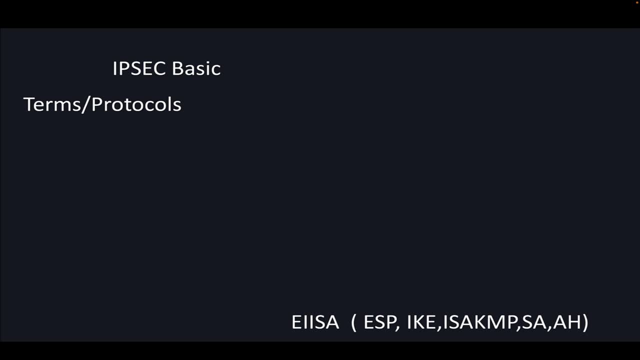 thing that I would like to point out is that if you want to send a message to the IPsec, that is the short form I mentioned, EIISA. okay, so what are these? so this is a little bit additional information you really need to know. ESP encapsulating security payload. this is used for confidentiality and 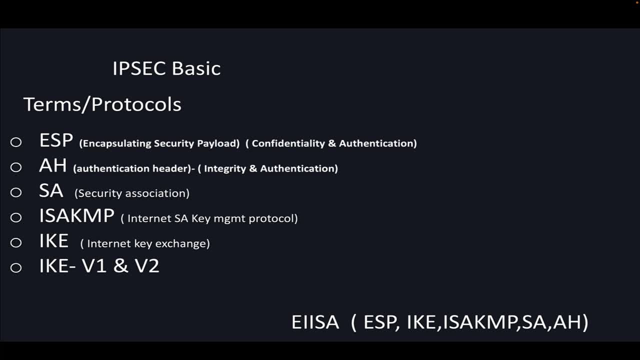 authentication purpose. okay, that's it. you want to know when phase 1 and phase 2 is up. then your data has to go from one place to another place. at that time you will see on the wire shard, all the packets are ESP packet encapsulating security payload. after that you have a edge. that's authentication header this. 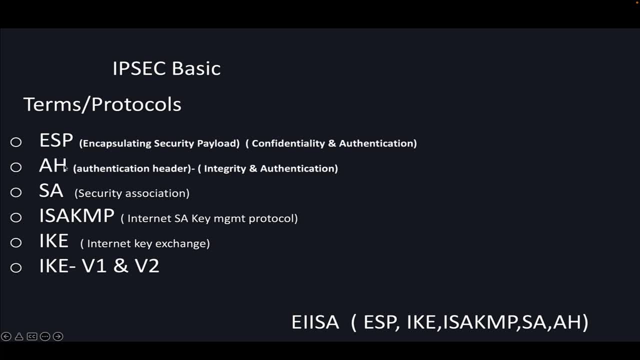 is used for integrity and authentication purpose. interesting thing to notice here is: in this we do not have any encryption like confidentiality. if you remember, that's for encryption, right, we do not get in the edge that what you can do, there is another way to use these both in the same way. so you can see that the 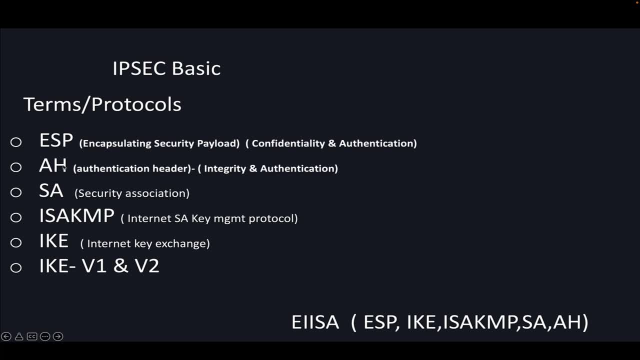 same way. you can use both in the combination like ESP plus AH. okay, because if you go into detail in a edge, there are some benefits of a edge, so you can use that. if you talk about the photograph firewall, you don't need to do anything. by default they are using ESP, they are not using edge. as for my 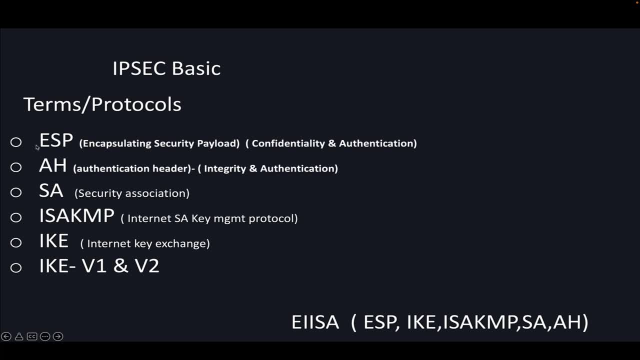 knowledge. maybe they are using, but as far as I studied they are using only ESP. then there is a security association, the head of information that we have shared with each other than the agreed. so that's called a security association. I say KMP. you have seen in wire shark there was I sick MP protocol. that is. 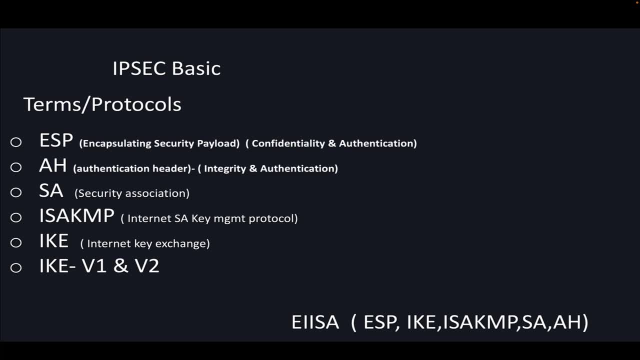 useful like Internet Security Association. key management protocol like this is for managing the key. you negotiate couple of the packets, all those packets are going from here and there with the help of, I say, KMP protocol. okay, so essay is the same here Security Association they do over the internet for managing the key. 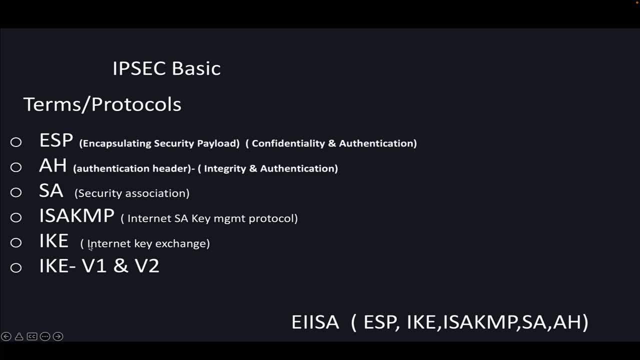 this is how you can remember that internet key and the key management exchange. so you have seen like we were using version one in that. if you don't remember, let me go back because here is like IKE, internet key exchange and there are two words on version one and version two, version like mostly I see still. 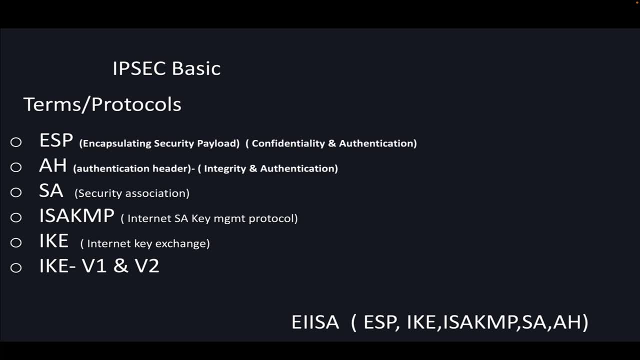 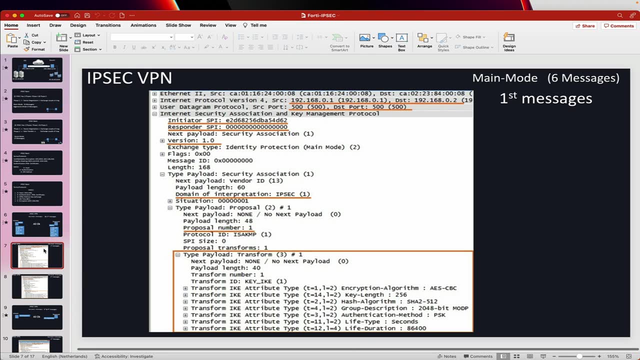 version one is being used widely, but version two is more secure. it's much better. there are a lot of benefits of version two. okay, so I would just say: you just use version two. you can see here there was somewhere- version one is being used. so this is the ice I person. these are the only things you need to know. 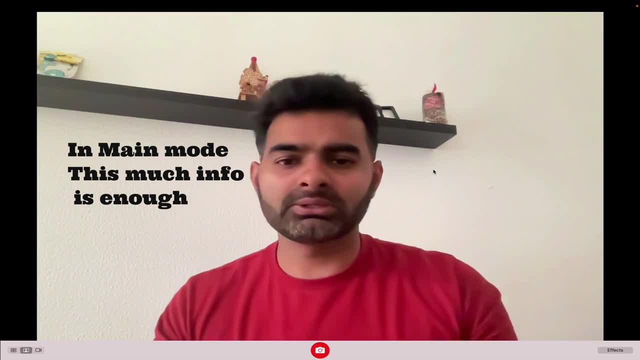 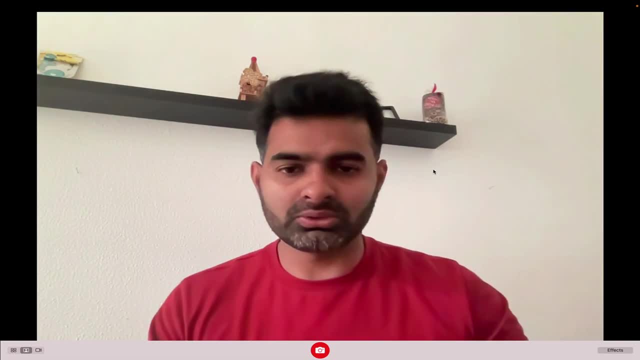 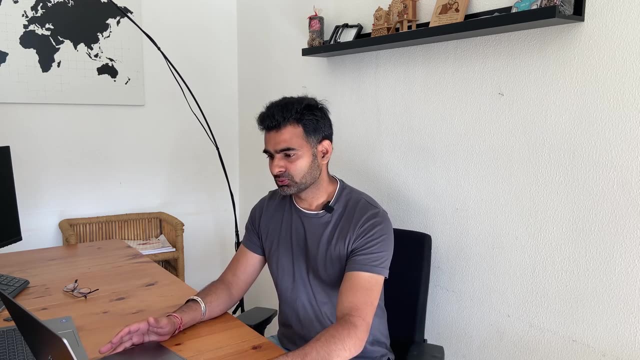 from inter perspective and also if you're working in a company. you only need to know these things. there is a hell amount of information on IPSec VPN. you don't really need to know into more detail. this is a part two of IPSec VPN. in this part, we will understand what is aggressive mode. so let's continue in. 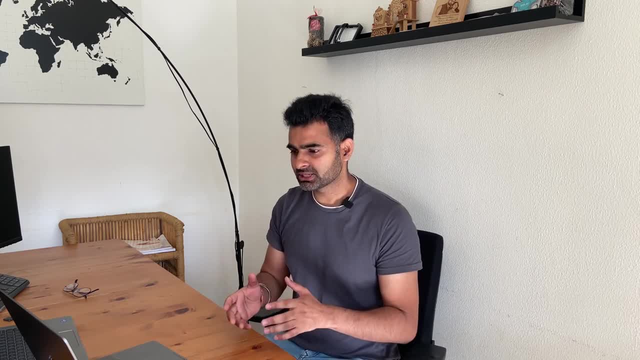 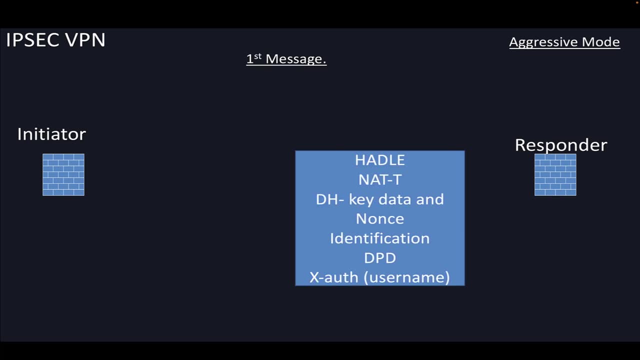 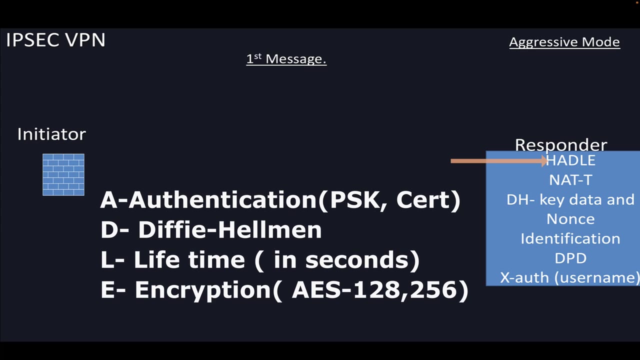 aggressive mode, three messages are exchanged. and let's understand what those messages are. we have initiator and responder. so in this, initiator is sending first message to responder. you can see in this we have hedl. we have understood what is hedl. h is hashing, a authentication default helmet, then L is lifetime and E is 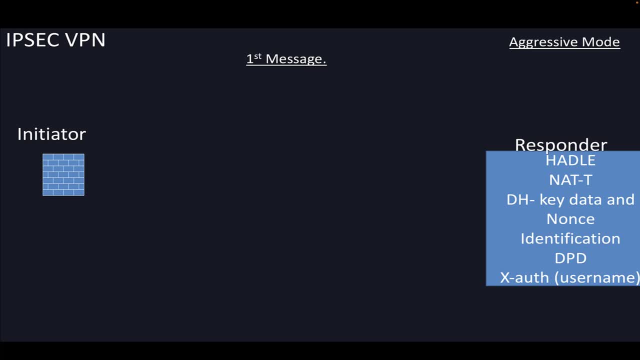 encryption. so this all information goes in the first message, but apart from that, the NATT also goes. DP haven't key data also goes and along with that, as goes the logo on this side of the message makes it easy to make a call, and also goes, and along with that as well, as we have a message that is an object of. 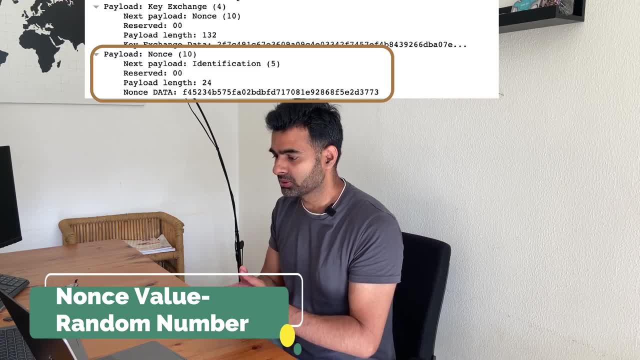 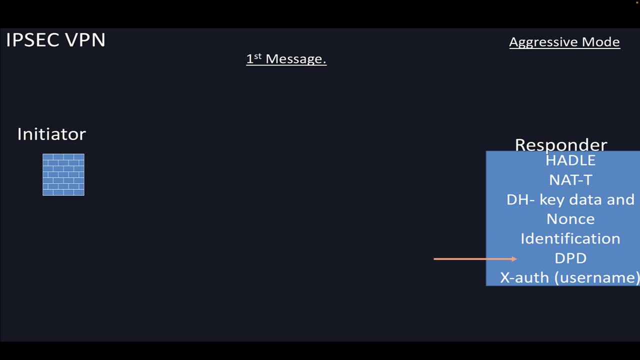 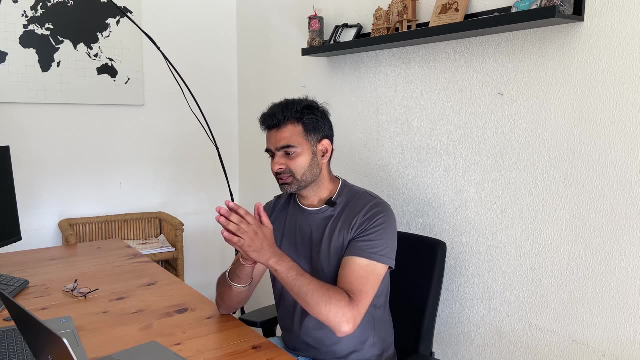 know in dphal, when nonce value is a random number, that also goes in this message and then identification goes off. initiator dpd goes dead. peer detection and x authentication also is a part of this message. from this you can understand that this message is equivalent to first four. 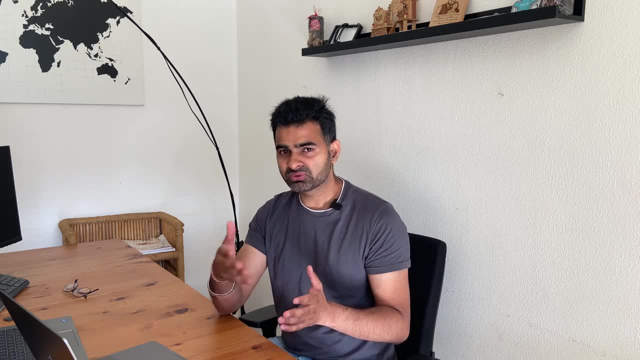 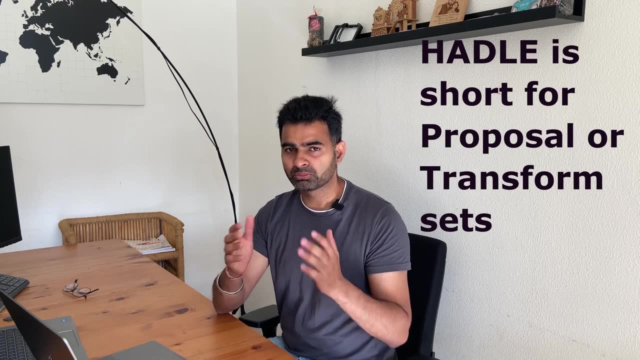 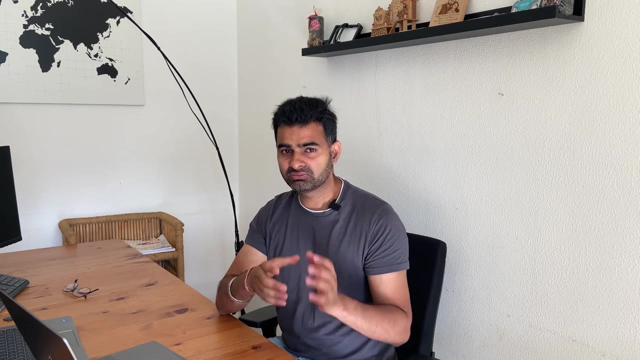 messages in the main mode, because in main mode in first message header information goes, the devices exchange header information and then they say, okay, we both support these kind of hashing, authentication etc. and in third and fourth message dphalman negotiation takes place, but in the in the 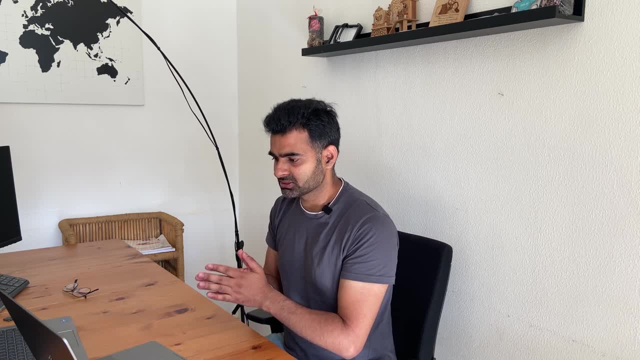 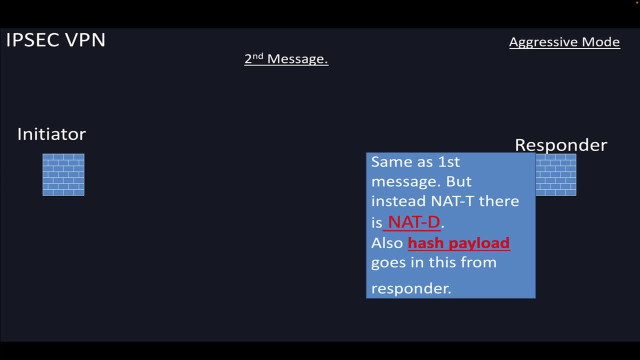 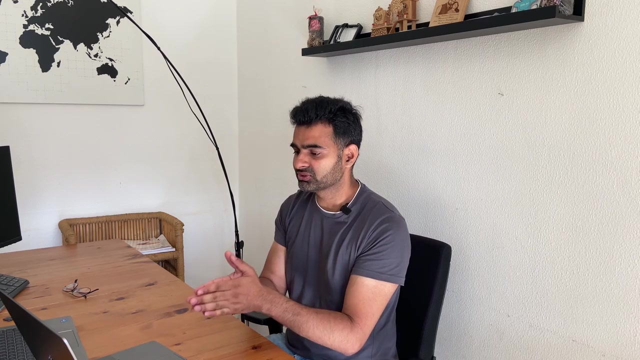 aggressive mode. that's happening in just first message. in second message let's see what goes in second message. exactly same information, what has gone in the first message, but apart from that, natd and hash payload also goes in the second message. hash payloads are of responders, so you might be thinking that we haven't seen the hash. 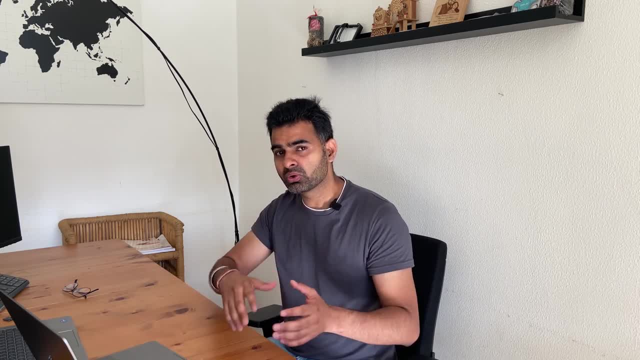 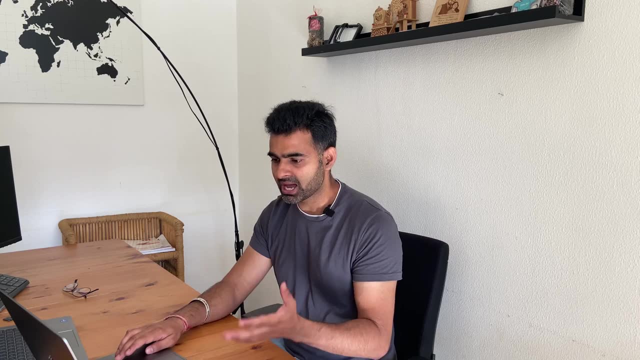 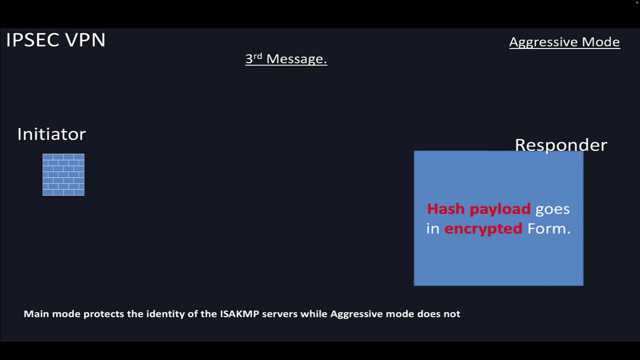 payload of initiator. initiator's hash payload will go in the third message. so here is, we have the third message. let's see. you can see hash payload goes, but this goes in encrypted form. the third message in aggressive mode is encrypted, so this is shared in the third message. 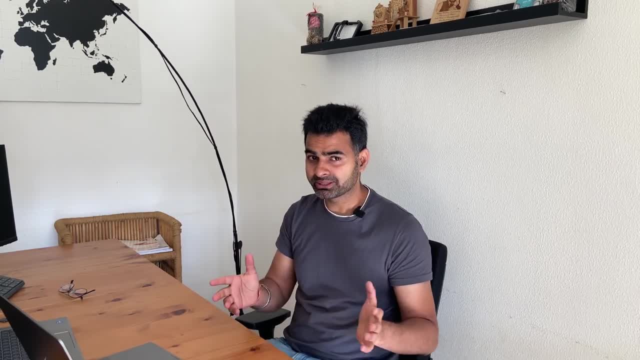 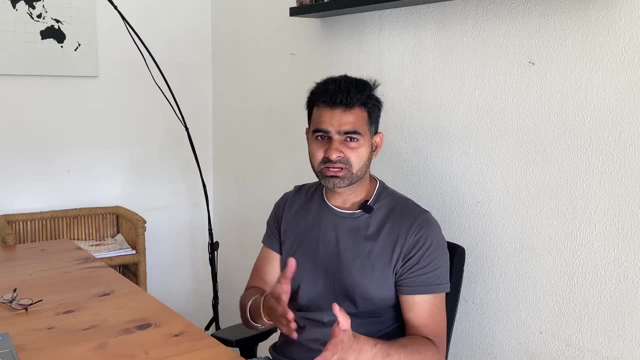 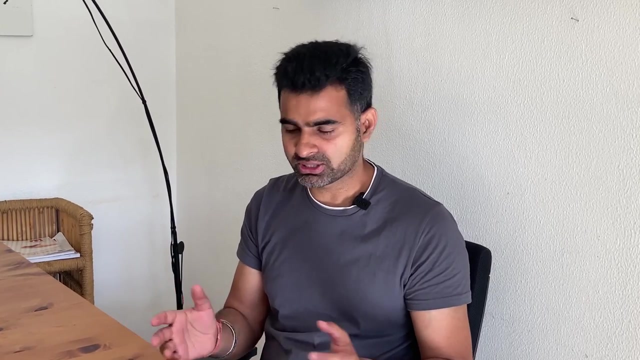 understood the main mode: protect the identity. however, aggressive mode does not support because in main mode fifth and sixth messages are encrypted and in fifth and sixth messages identity goes. this is very important exam question also and this question is also asked in interview many times, so please keep that. 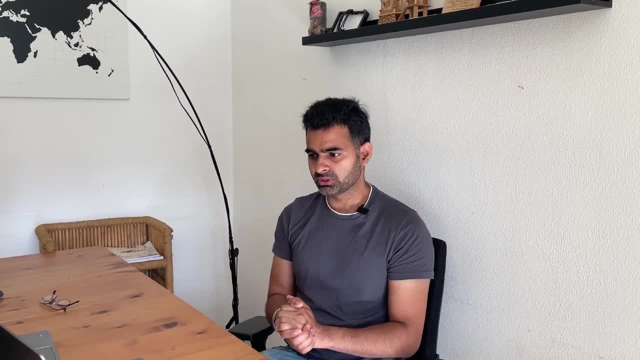 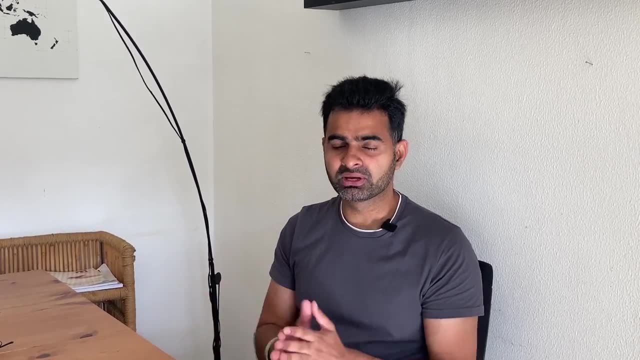 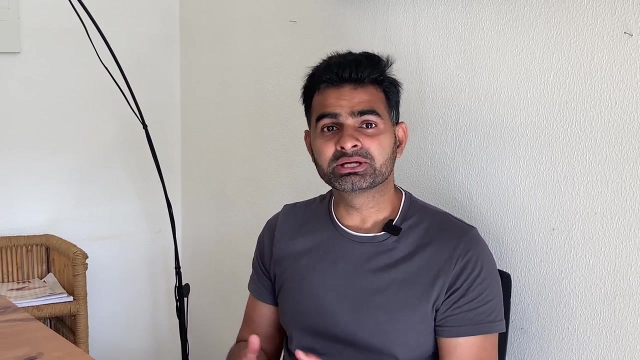 in mind. so what is the key takeaway from this video? is that you understood that three messages are exchanged in aggressive mode. it means it is faster, three messages are exchanged, but we also understood that identity is not encrypted, so it means it's not secure. it is fast, but it is not secure. the 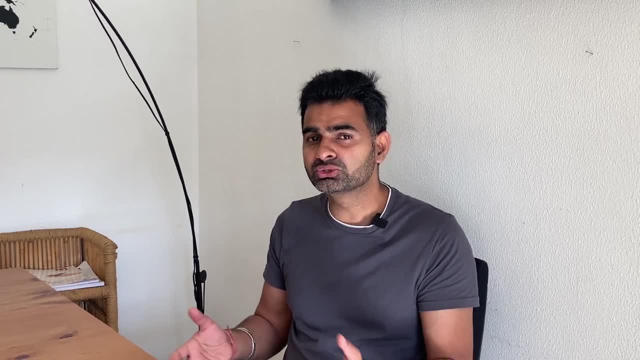 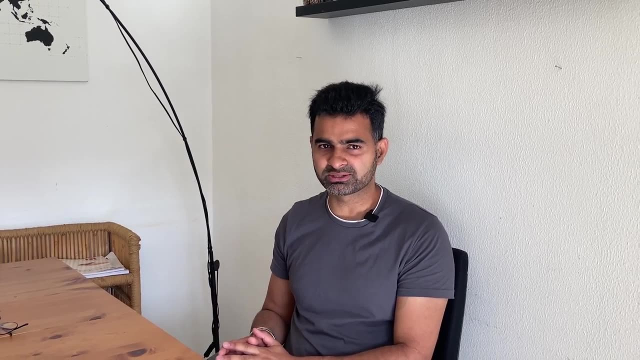 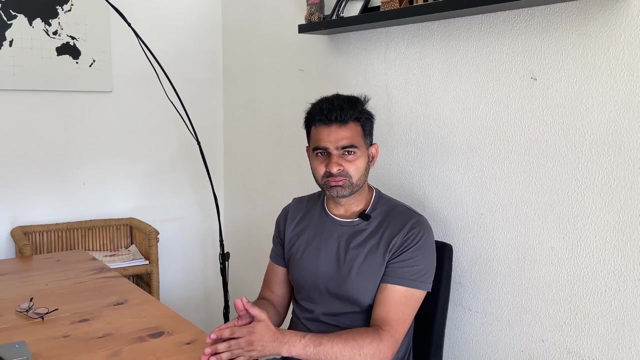 question is then why we should use aggressive mode or where we should use aggressive mode. do we still use aggressive mode because it is not secure? the answer is yes, we do use aggressive mode, and where we use the aggressive mode, we use the aggressive mode where you have to configure remote VPN for the people who has to work from home. 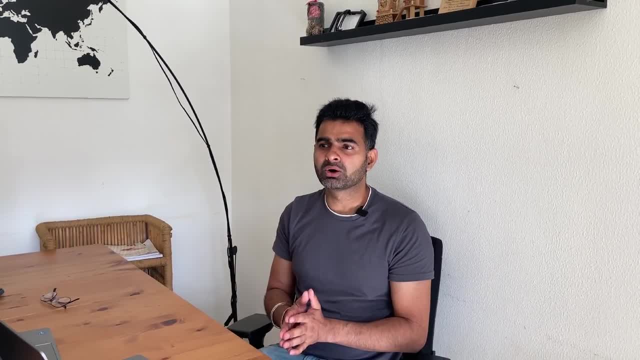 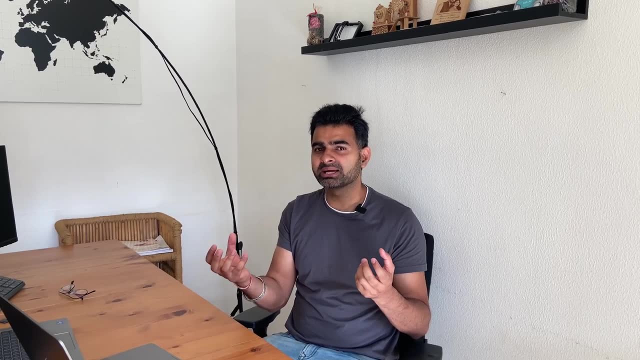 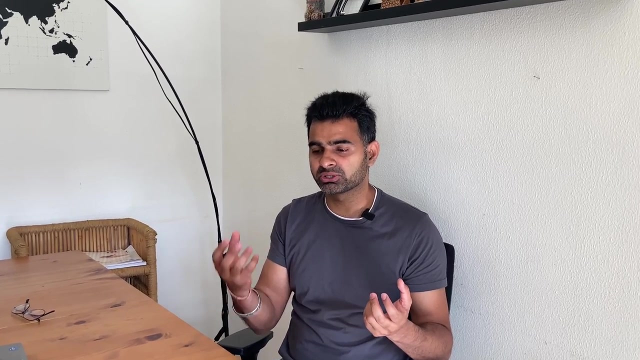 for them we use aggressive mode. and also if there are two sides and you have to configure the site to site VPN and one side has a dynamic IP address, its IP gets changed all the time. in that case also we use aggressive mode because the IP of this device will change. we cannot configure this IP in another firewall. so 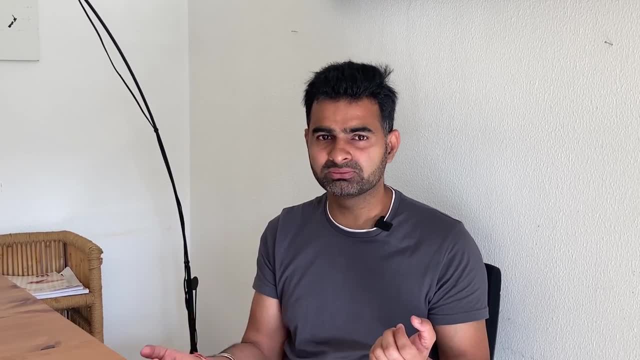 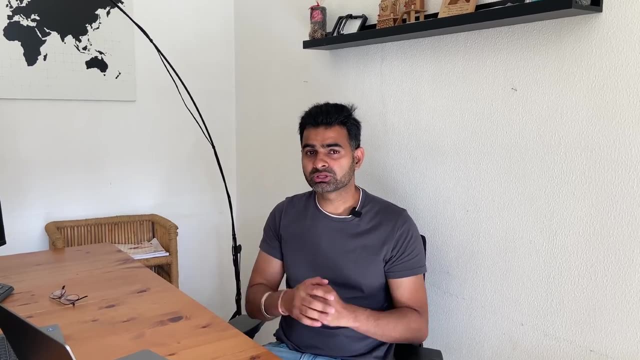 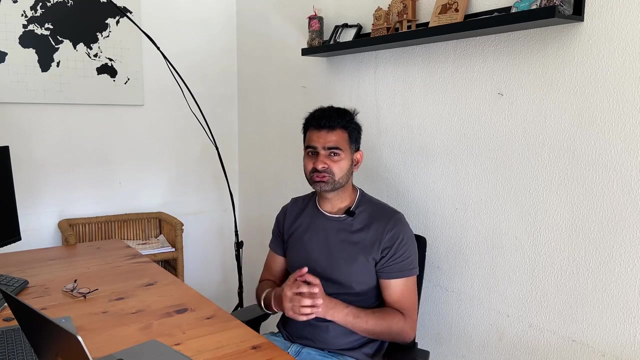 this fire. we're always act as a dial up, so it will dial the vpns and the process will start. so in these two kind of cases we use the aggressive mode. i hope you like the video. this was a theory and in my next video i will show you everything what we discussed in the world. hi guys, in our last video we have 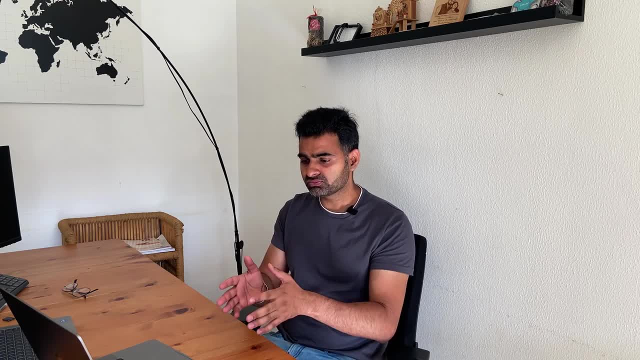 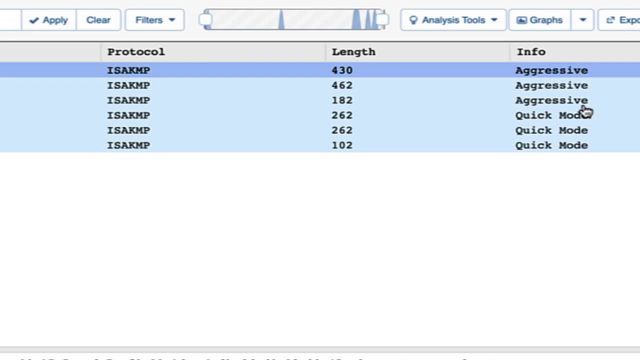 understood aggressive mode theoretically. uh, in this video we will see all of those things in the wire chart, so let's continue. you can see we have aggressive mode- three messages, as we have discussed previously, and then we have a quick mode- also three messages, but in this video we 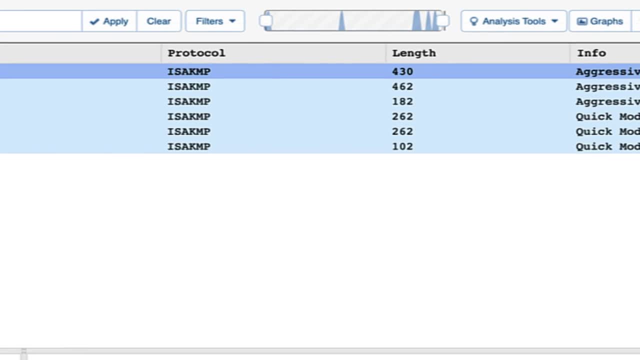 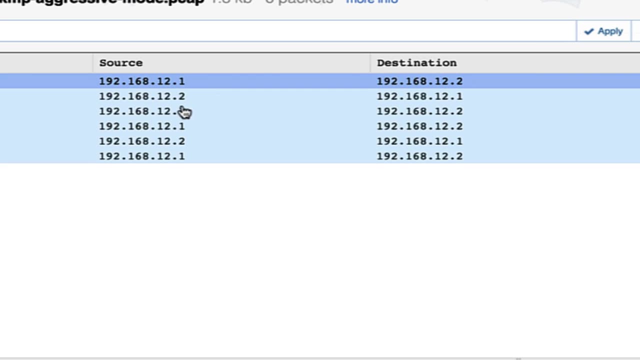 will only discuss about aggressive mode. first thing, you have to notice that 12.1 is uh initiator as source and it is replying to 12.2 and then 12.2 is replying to 12.1 and then 12.1 is replying back. 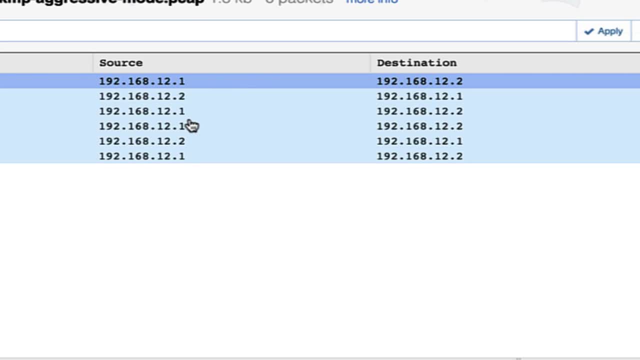 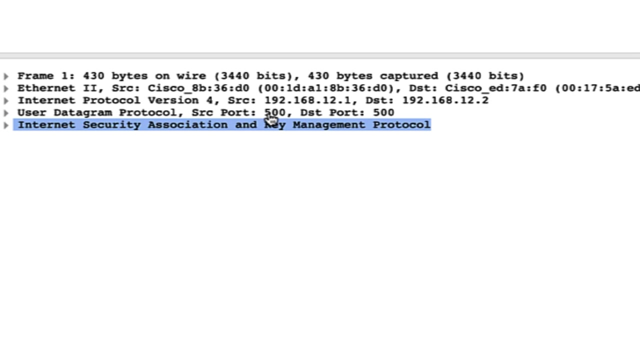 okay. so this gives you understanding that it's not the only first message. they keep changing. so it is: uh, three messages get exchanged. but don't make conclusion from here. let's go into a little bit more detail. another thing that you will see: uh, your ip, sec, isa, kmp, that gets exchanged over port number 500. okay, and another thing. 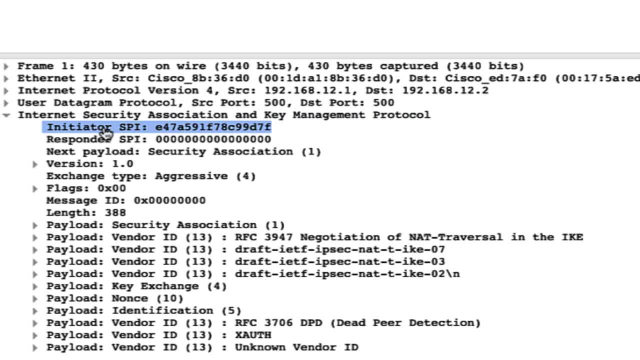 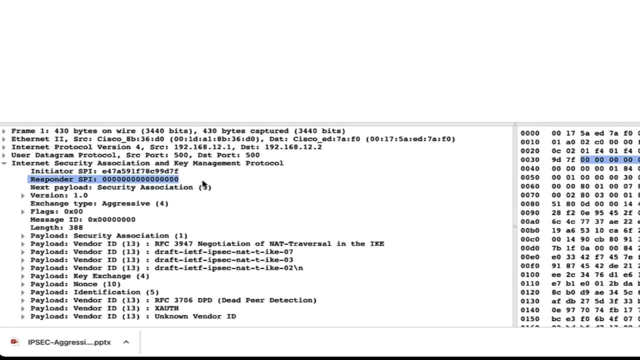 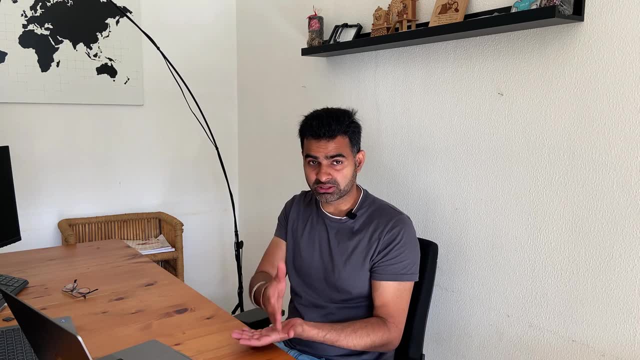 that we have to notice is because this is the first message. initiator spi will always be there because source is sending the packet, but responder spi is always zero, zero. so this is really a that will be asked in interview: how you will identify first message in aggressive mode. 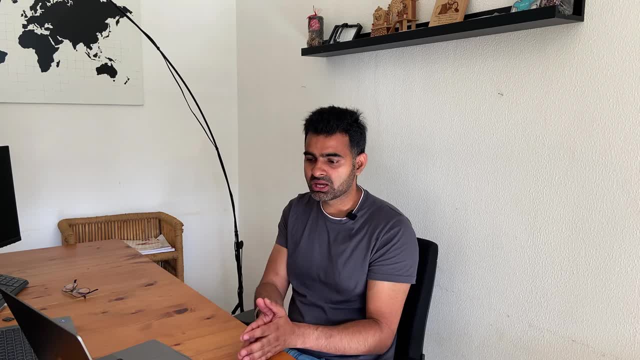 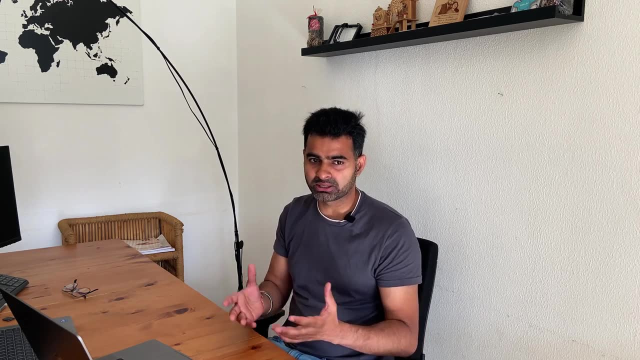 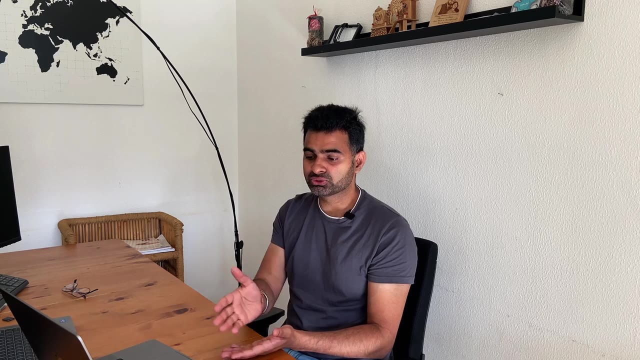 are in the main mode. so you can say in the first message, initiator spi is always filled. however, responder spi is not there because responder has not yet replied. okay, and then let's go. what's there? here we have the version. uh, we are using ike version one. 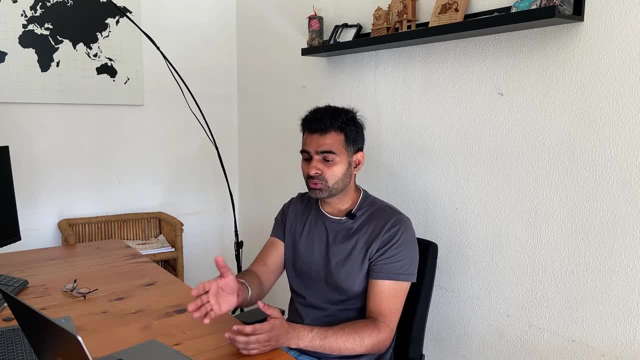 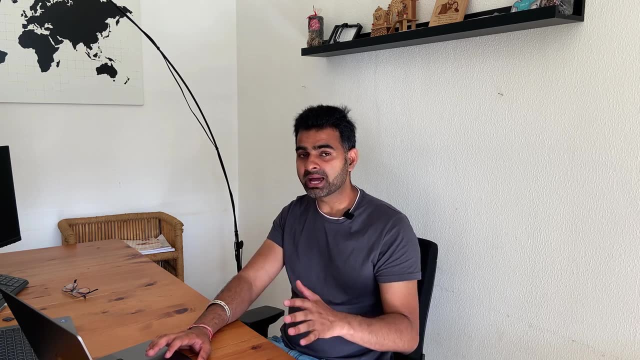 and in that we are using aggressive mode. if you would be using main mode, you will see that here. this is ike version one. in ike version one only you have aggressive mode and main mode, but in ike version two you do not have any kind of main mode or aggressive mode. we will discuss that in our 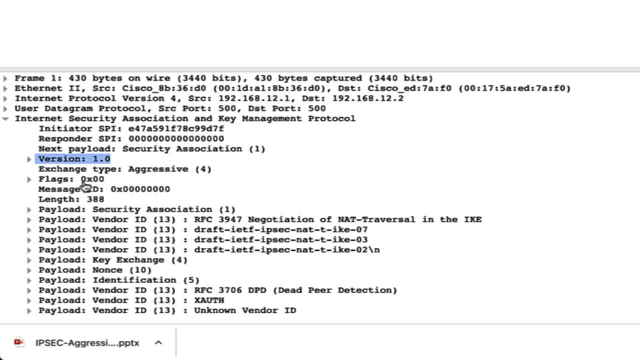 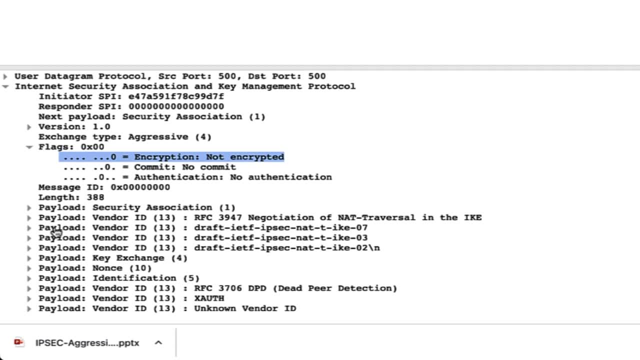 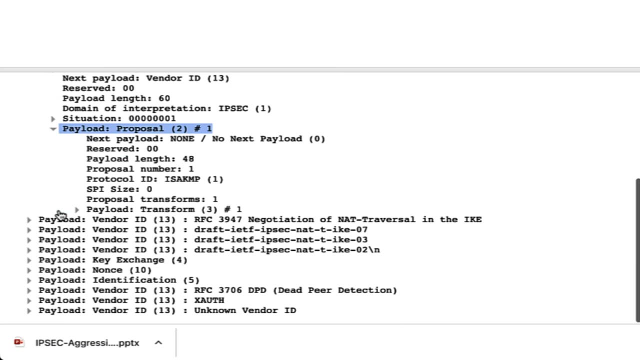 different video. okay, so let's go to the next flags. this is really not interested. only thing you can see, like this is not encrypted. of course we know this is not encrypted. that's why we are seeing everything here. nothing is encrypted in the first message and let's see a payload proposal. okay, this. 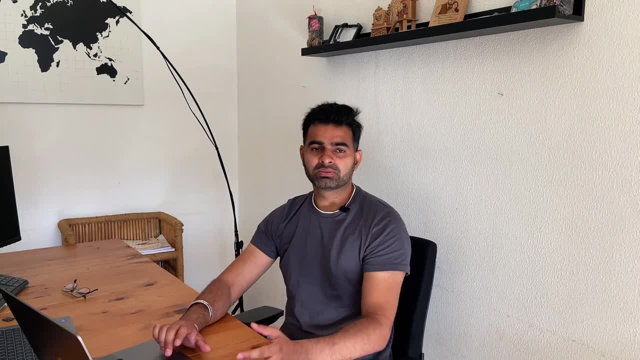 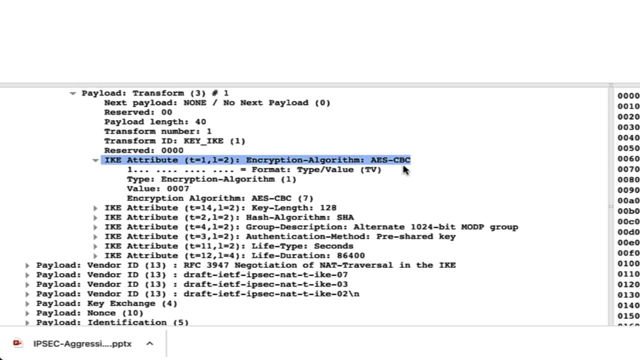 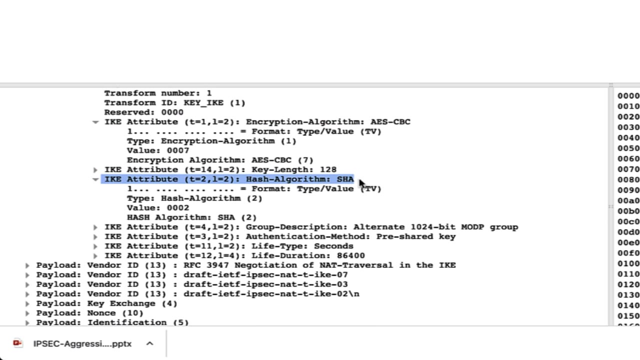 is interesting. so this is the header information that i have told you. so what goes inside that encryption? okay, which encryption? we are using, aes, cbs encryption we are using, and the key length is 128, which is secure. uh, then you are using hash algorithm as a sha, sha2 and group number. we are 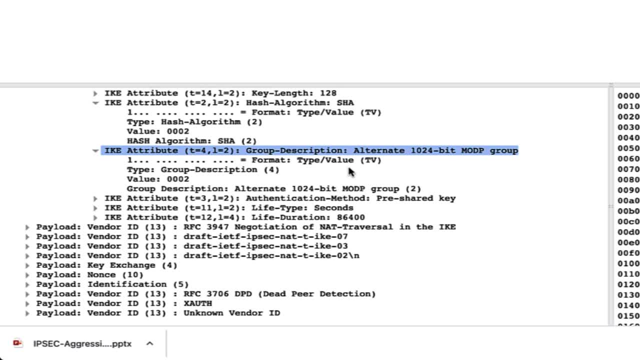 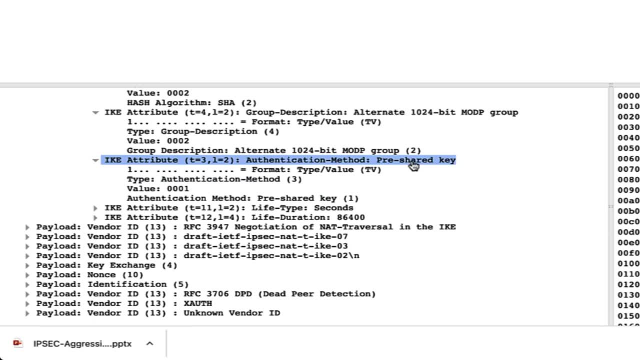 using is one, zero, two, four bit. uh, we are using uh, but the number is four. so, um, but if you want to use the password properly, and then you will see here: pre-shirt key, we are using pre-shirt key. we are not using digital certificate. another thing i want: 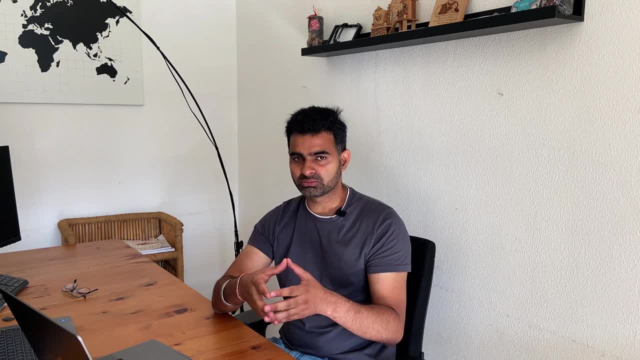 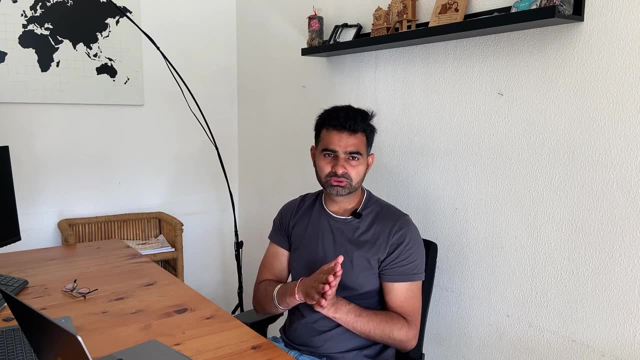 to tell you, if both the hosts are using digital certificate, you don't need to use the aggressive mode at the time. that's also an exam question, okay, because digital certificate will never change. we uh have understood in our last video. if there is a dynamic host, if there is a device which is getting 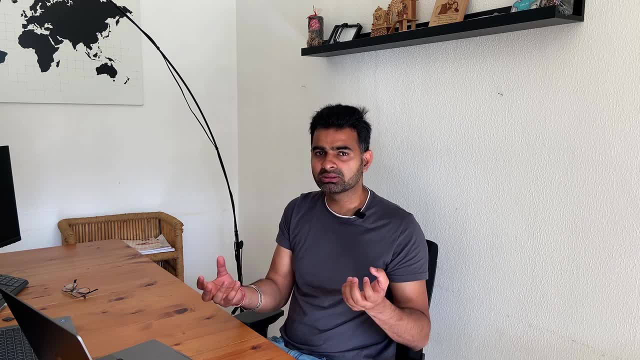 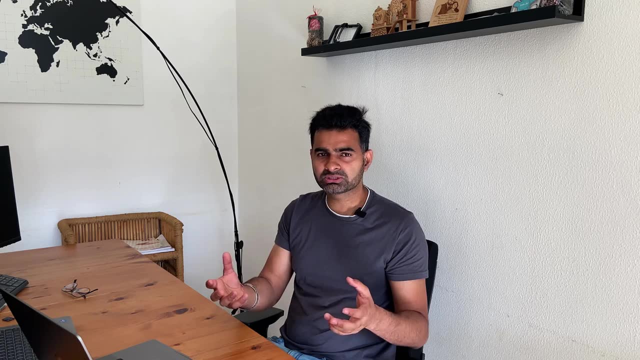 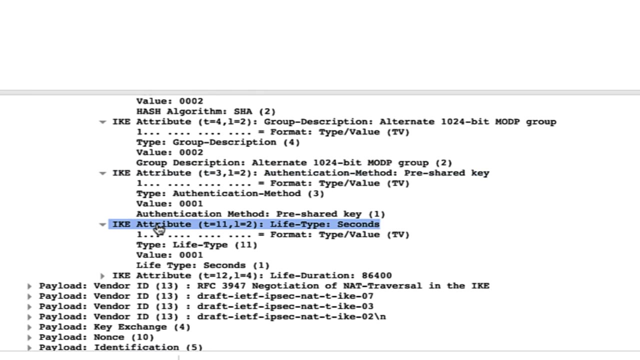 ip address dynamically, so its ip keeps changing right side-to-side tunnel in other side, like what is the IP address of the remote, and so it will always dial up. in case of digital certificate, certificate will never change. it will be same. so in that case you can just use main mode, okay, so? 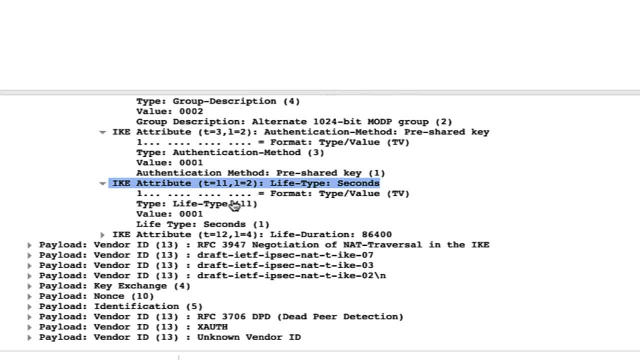 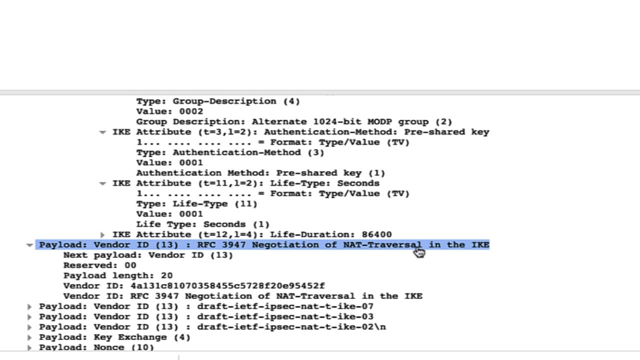 what's the next? next is a lifetime which goes in the seconds. so here you can see how much lifetime is there: eight, six, four hundred. so we have all the information of Herald and we have discussed that. in first message NAT traversal goes, and in second message you should see NAT detection. okay, so they. 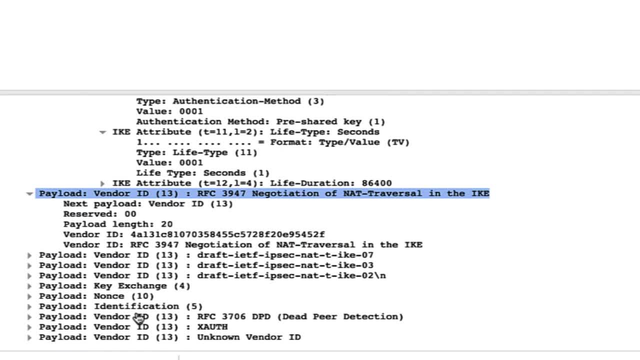 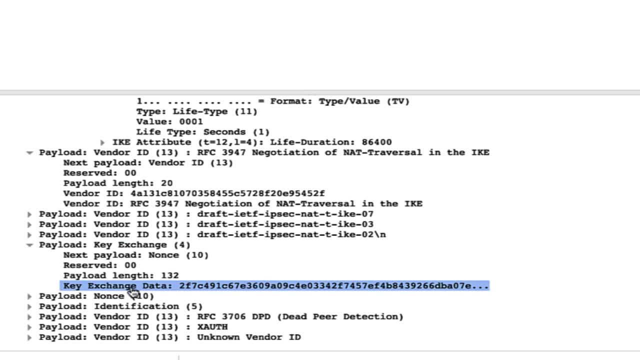 said: okay, we will use NAT traversal, and they detected the NAT, so that goes in the second message. so they all are NAT T package and then this is a key exchange. so this is a Diffie-Hellman. I told you that key exchange data is sent and also. 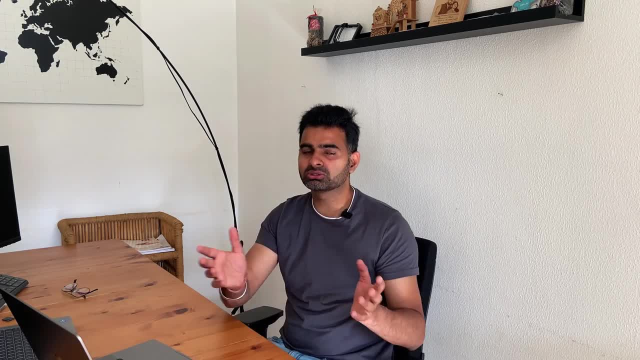 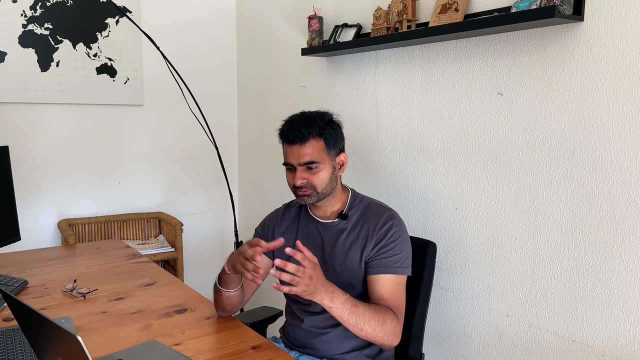 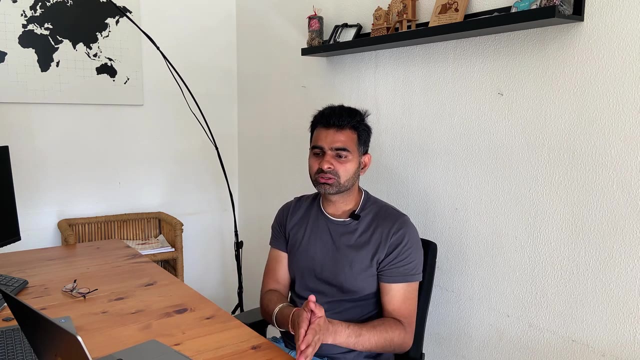 the NUNS value is sent. so these two information goes. this is also exam question. they can ask what information goes. when I'm saying exam, I mean interview. I don't know why I'm a habitual saying exam. this is really an interview question and I myself also asked this kind of question. what goes in the third and fourth? 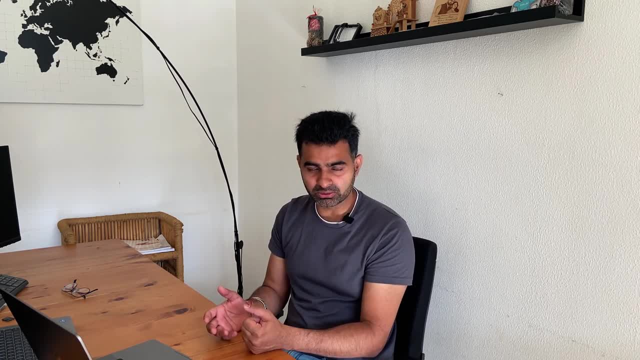 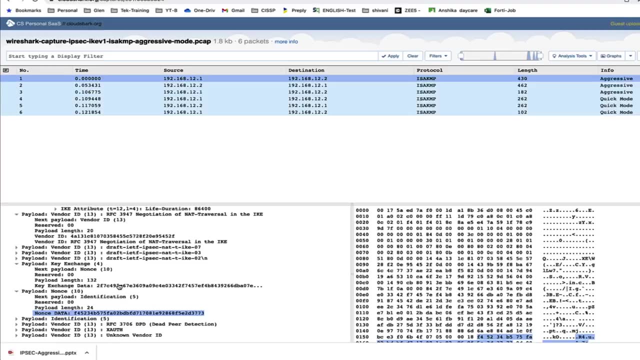 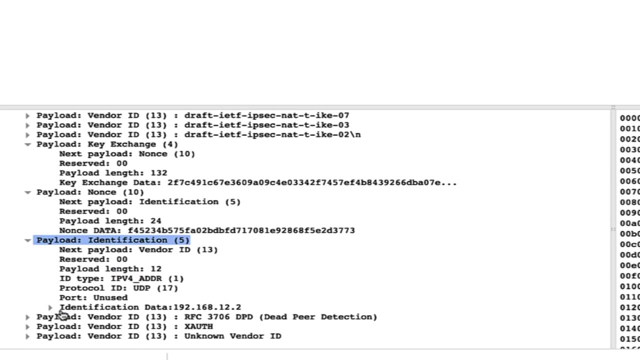 message in main mode: okay, what goes as part of a Diffie-Hellman negotiation- you can say key exchange data and NUNS data goes as part of TH negotiation. okay, and you don't really need to remember this number because these are just random numbers number, so they will keep changing, okay. and then there is a identification. in identification most. 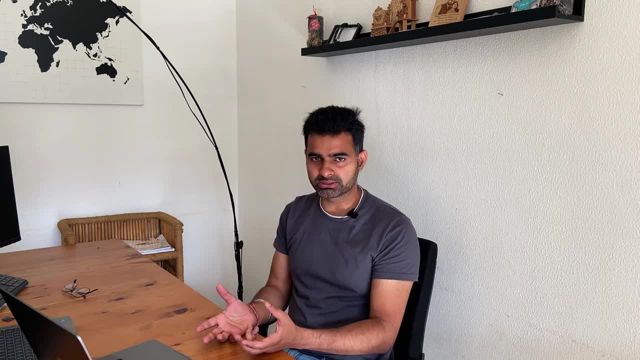 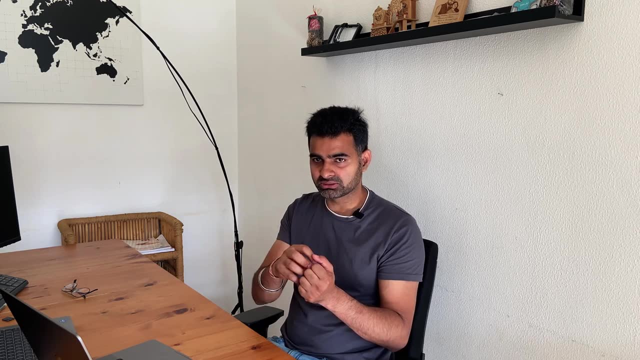 of the time, identification is always the public ip address means the van ip address, because the external van ip address is the ip from where you will initiate the tunnels right. that's the reachable ip address. so most of the time it is that, but you have the option to put. 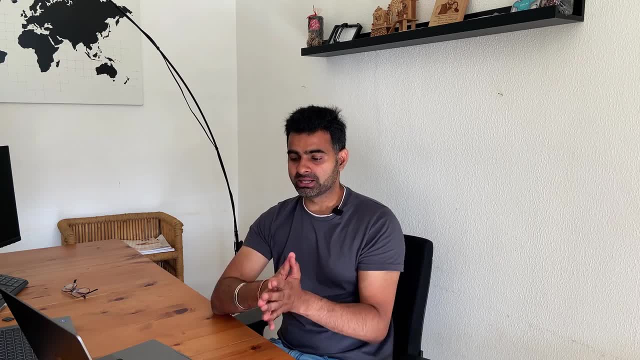 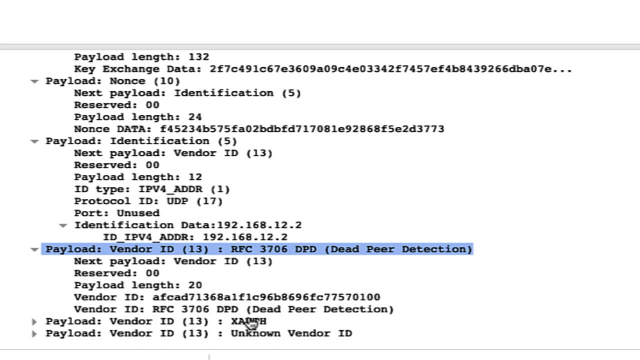 the peer id and remote id. if you will put the peer id and remote id that you will see here, okay, and then you have a dpd dead peer detection- i also told you that it will go there dead peer detection- then x authentication will go there most of the time. in x authentication, username is: 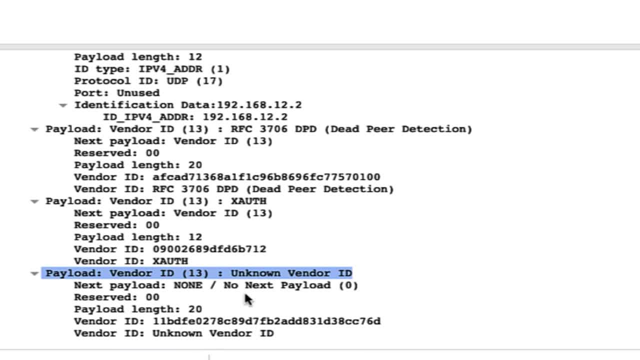 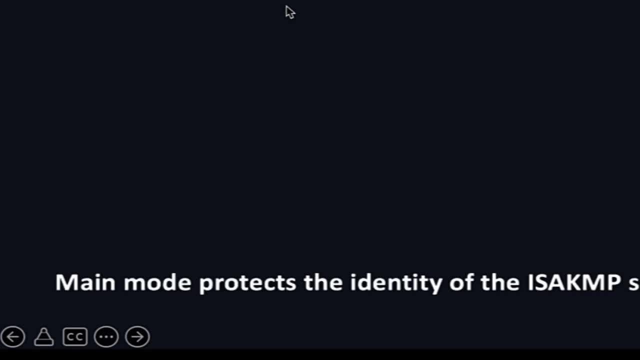 there? okay, and then what is this payload vendor? okay, this is all the information we have discussed in our previous lecture. let me go back and show you that i think here, so you can see. uh, this is second message. we have not yet read that, so this is all information. handle nat t if you. 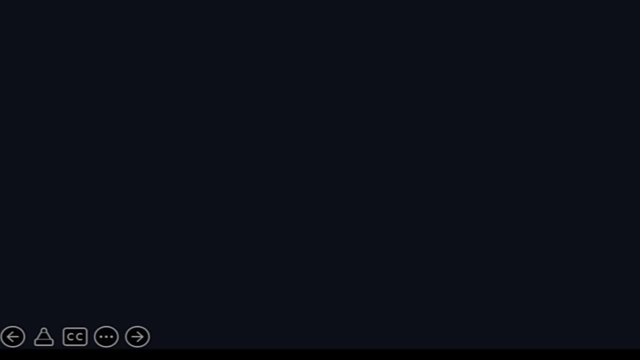 help me: nuns identification, which was ip address, dpd, deadp detection and xauth. we have seen all of these things in the washer. let's see what is in the fourth message. if if i show you my slide, i shown you everything. what was in the first message goes, but instead of nat t, nat d goes also, you will. 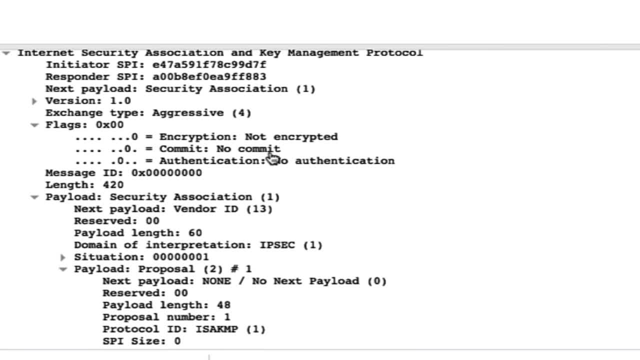 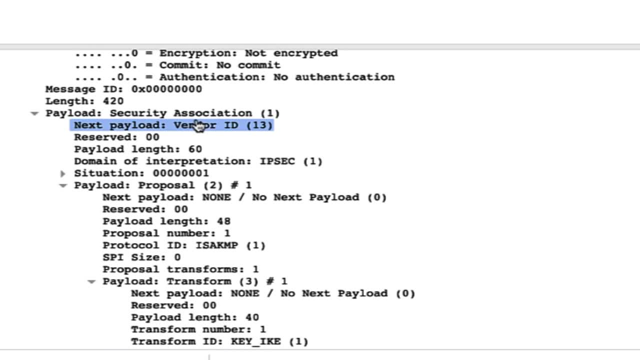 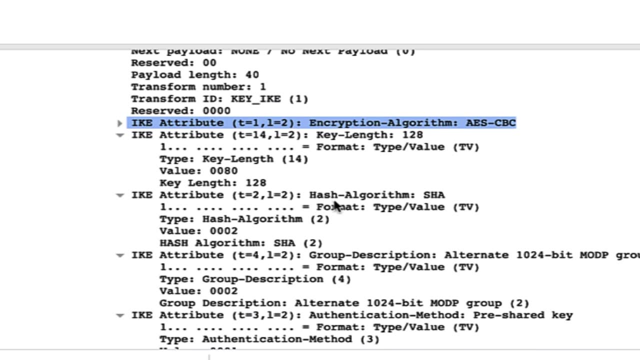 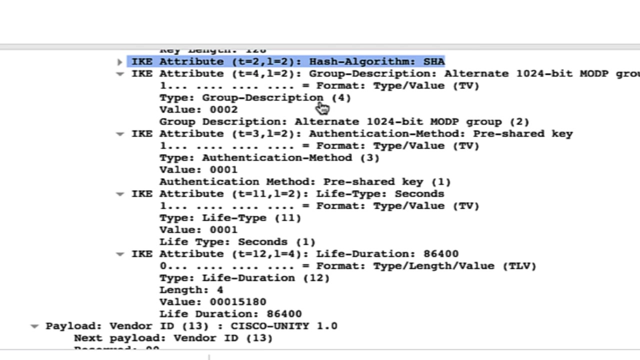 see hash payload here. let's see, uh, what we will see here. okay, so version is there. okay, we are using aggressive mode and, as part of the security association, we have some proposal. let's see where they are. they are here. see encryption: same encryption, same key. so we are using sha 2 and shadow is here. sharp, we are using and the. 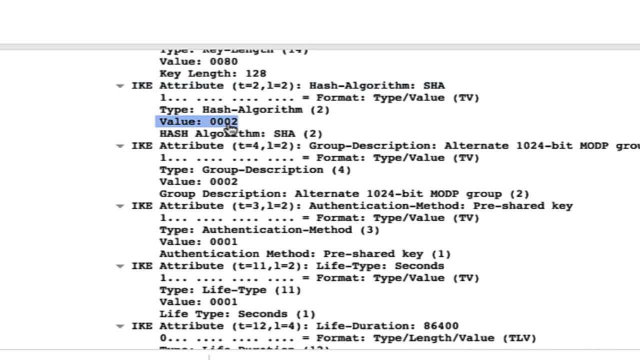 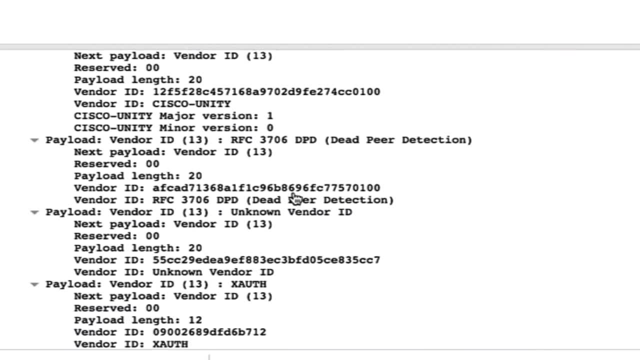 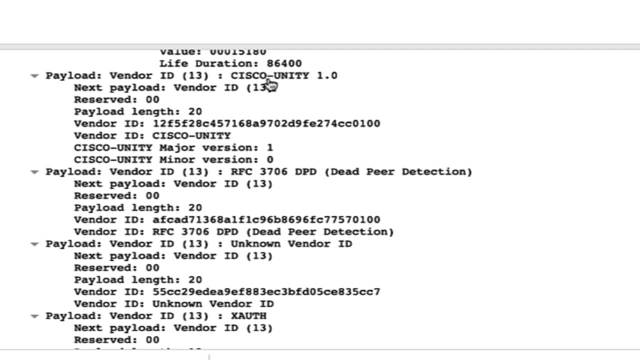 version is 2, but it got minimized when i click uh, okay, sha 2, and then you have a group, okay. so you can just see all those things slowly by pausing the video and what else goes in that you can see that the uh, the version is also going. this is probably the cisco's client. 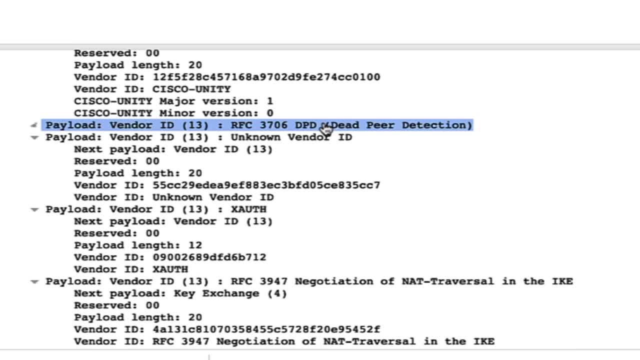 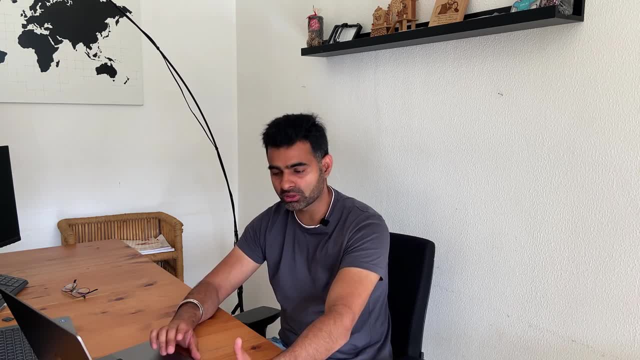 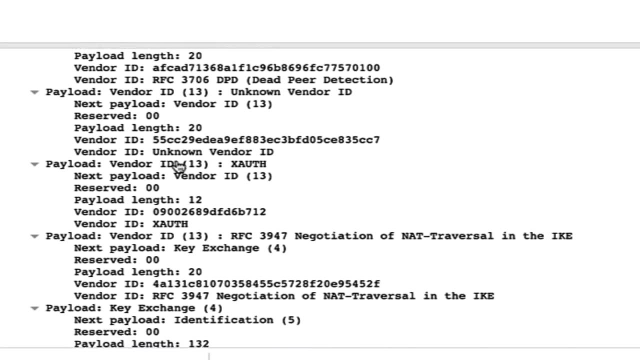 and the next thing is: uh, dead beer detection. okay, that goes there. definitely, both beer has to negotiate if they are that dps enabled or not. okay, if the peer is down, they have to detect each other. and then, uh, what is this? this is nothing interesting. then, xauth is there. uh, what else you? 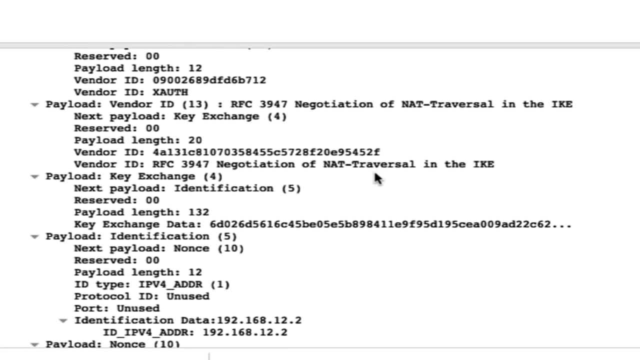 can see nat t e um. yeah, so this is the proc, municipals agreement, net fon the two. i'm going to do copy and paste version of this and then stay on the speaki as dedicated history. so this side. so so traversal is there, but we should also see NATD. I hope I am in the second message. okay, so NAT. 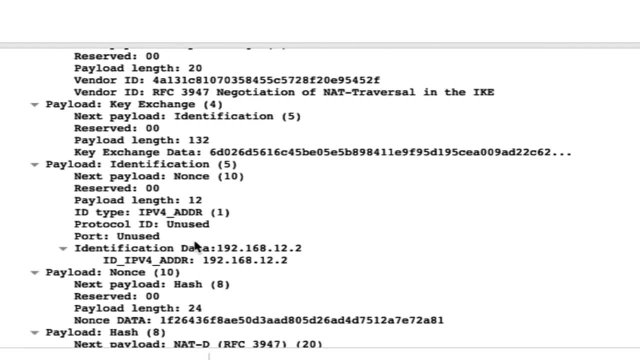 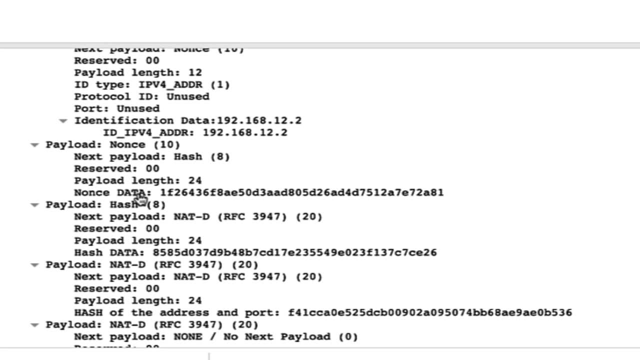 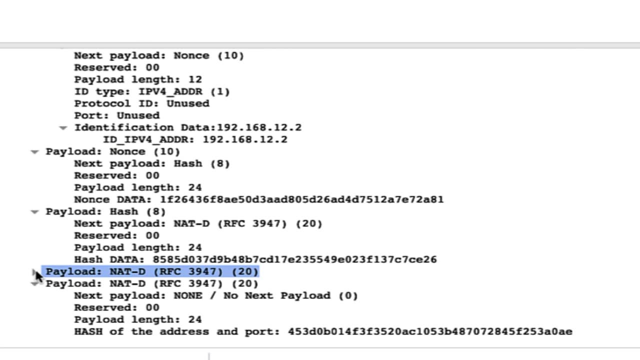 traversal is here, NAT travel is here and identification IP address is there. okay, here is our hash. so the hash data is going. that's what we discussed. hash payload goes here and here is your NATD, NAT detection. that's what I told you, right? so, if you, if I go back, NATD and hash payload. 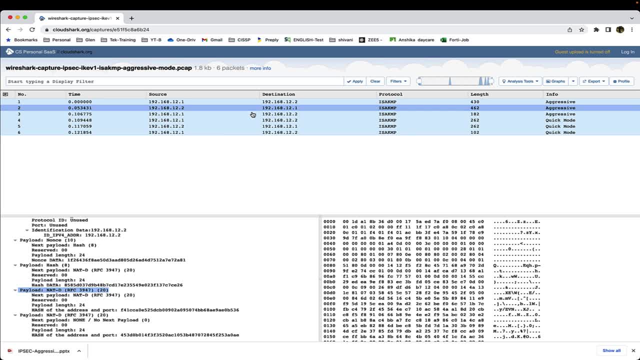 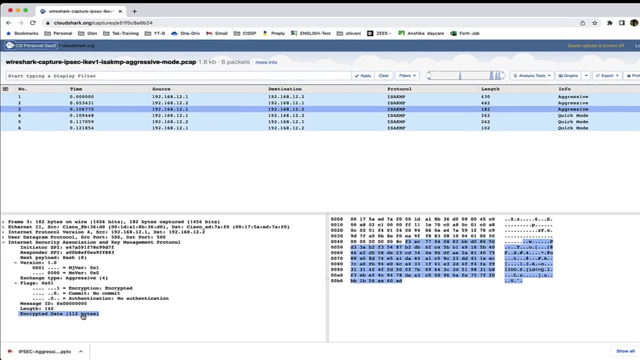 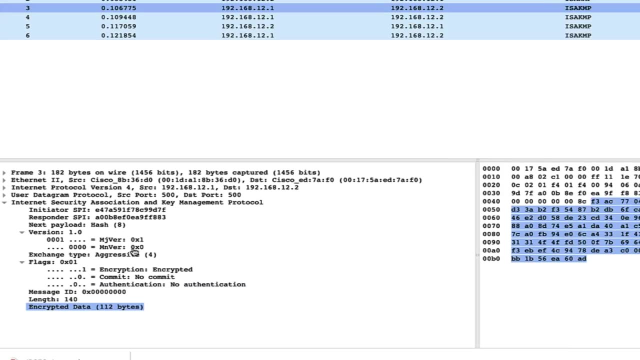 are the additional things that goes in the third message. sorry, second message. third message is magic. you don't see anything in this because this is encrypted, right? so see, this is encrypted. authentication, no authentication. this is encrypted at all. you cannot understand what's going inside that. so, theoretically, what goes inside that? where is my packet? 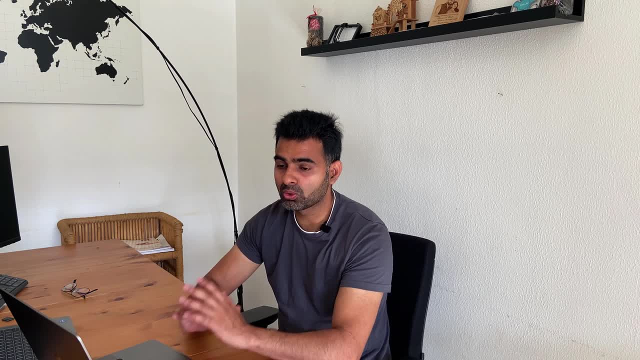 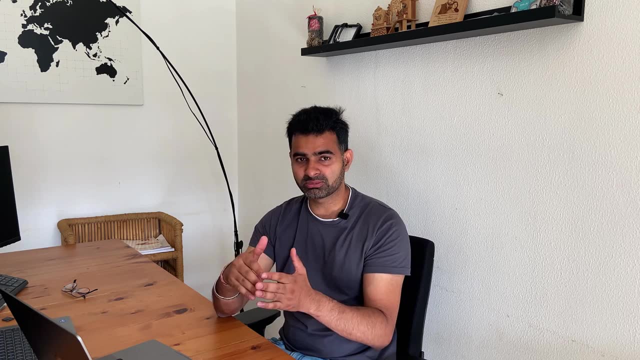 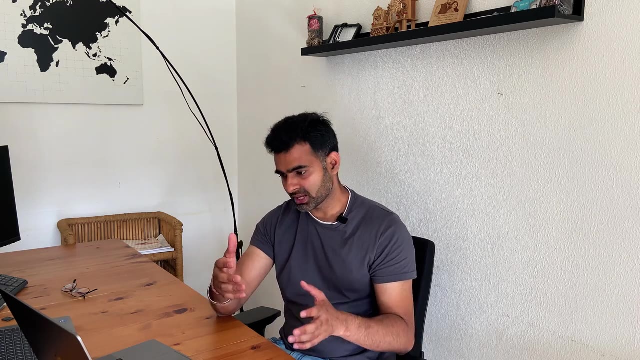 hash payload in encrypted form. whose hash payload? initiator's hash payload? because the initiator never send the hash payload in the first message he never sent in second message. responder sent his hash payload in third message. the hash payload of initiator will go in encrypted form. that's it. 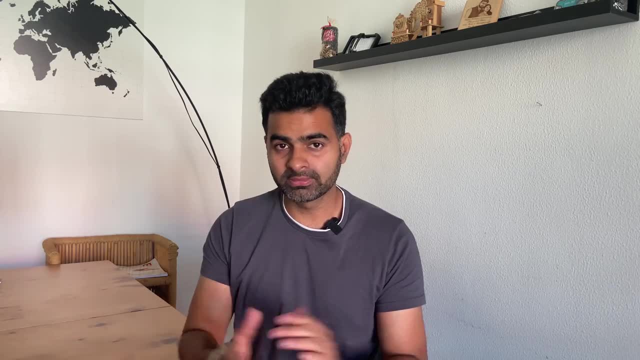 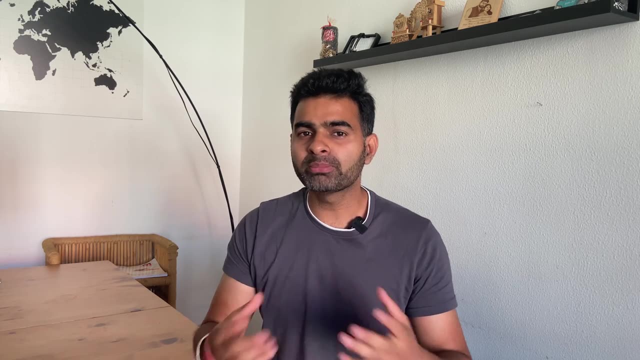 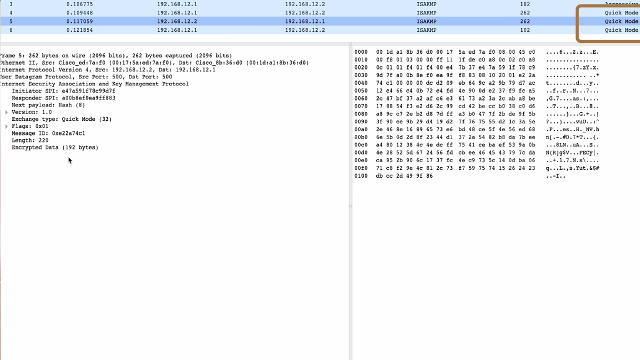 in the next video where we will discuss the quick mode. hi, in today's video we will discuss about the phase 2. in phase 2 we only have one mode and that is quick mode. all the packets of phase 2 are encrypted, so there is not much interesting to show you of all those packets, but we will understand what goes in. 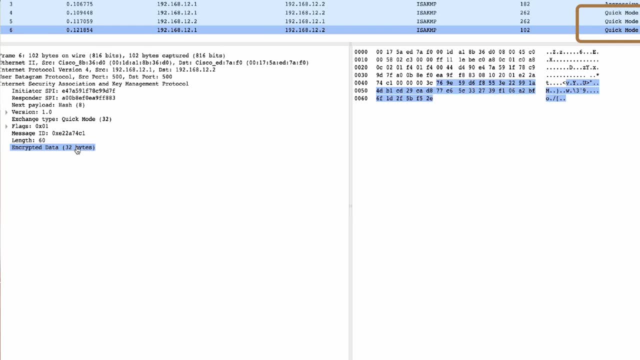 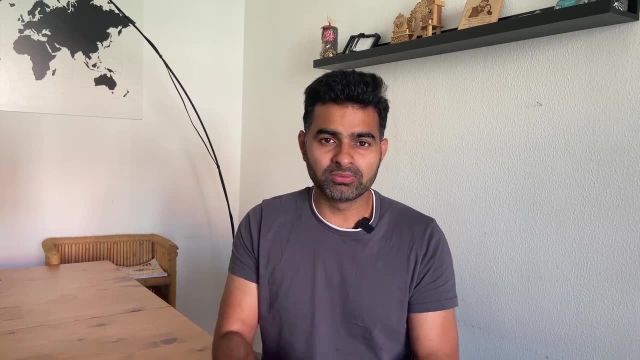 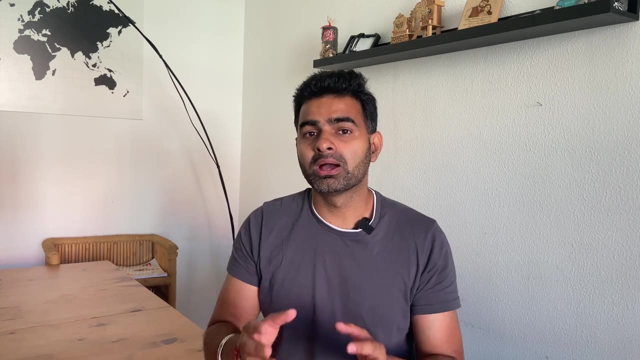 those packet. before understanding that, let's understand why those packets are already encrypted, even before they have shared all their handle information and how they are encrypted. if you remember, we have already established the phase one tunnel and in that phase one tunnel, as part of message three and four, uh, we have negotiated diffie hellman. diffie hellman has helped us to. 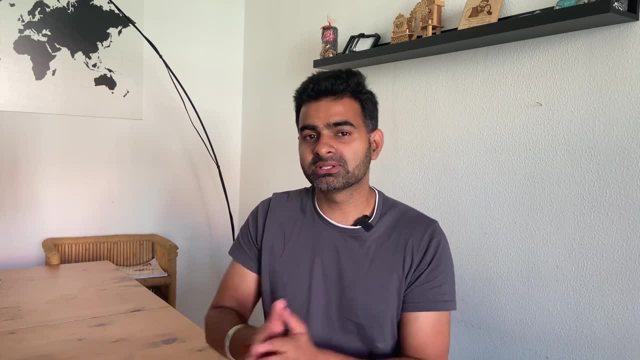 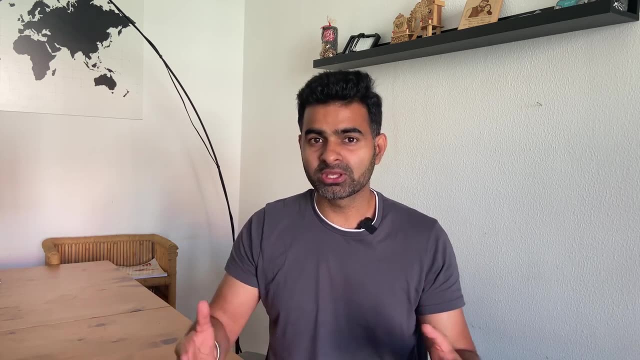 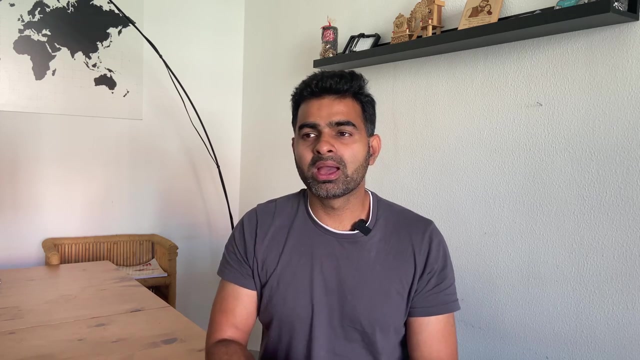 create a shared secret key and with the help of that, the fifth and sixth message was encrypted. phase two goes inside the phase one. that's why it is encrypted, so you can understand how secure it is, like tunnel inside tunnel, right? so that's the one thing, and now let's understand. 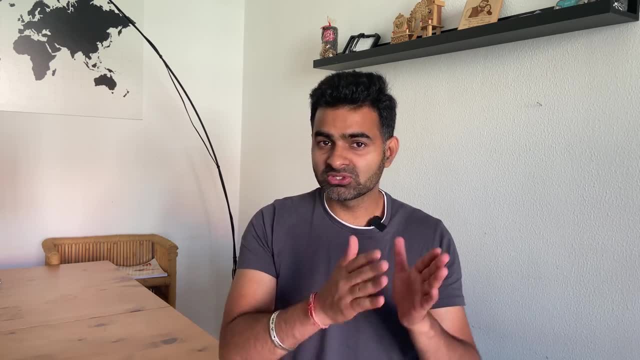 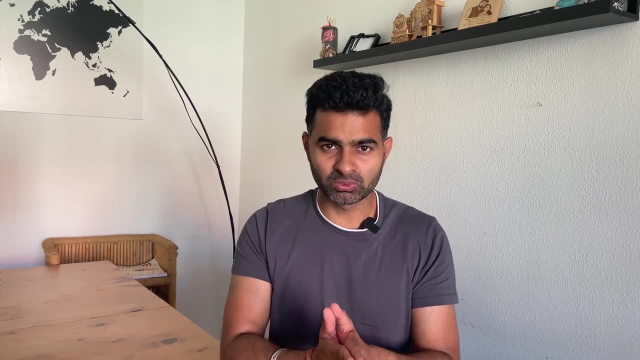 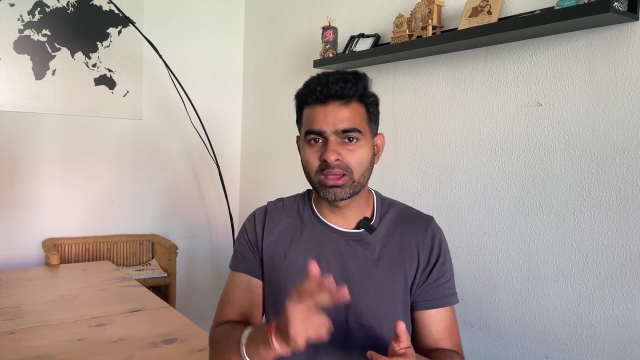 what things goes inside that. uh, in the first message which is sent by initiated to remote host- remote host- we will say the responder and the first message: security association will go. you can also say security proposal will go, or transfer and set will go. in that you have your hashing algorithm, you have your encryption algorithm, you have your. 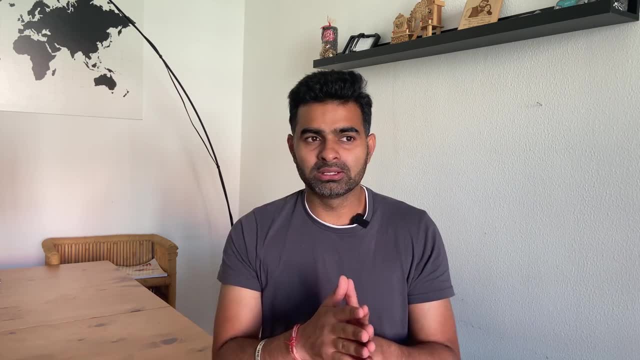 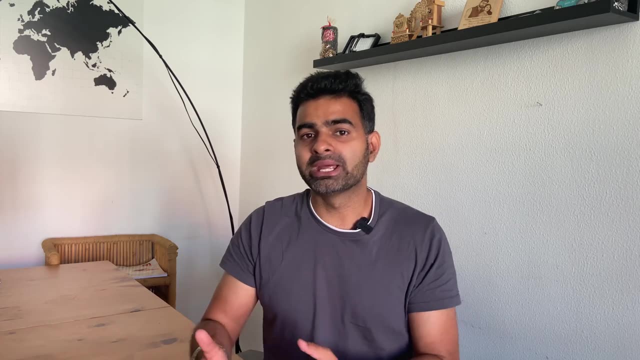 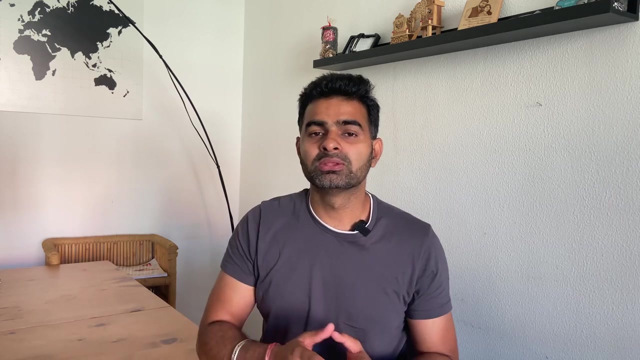 Diffie-Hellman group mentioned in that, and your lifetime will go that, after how much time you're at home, how much time your key should get expired. there are some other things that also you can enable. you can enable PFS perfect forward secrecy. there's another option that you can enable as part of phase 2, that is: 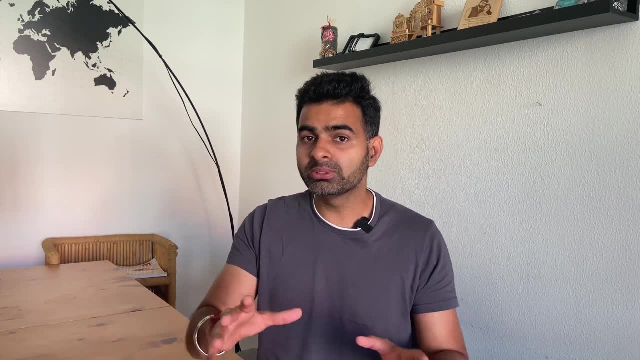 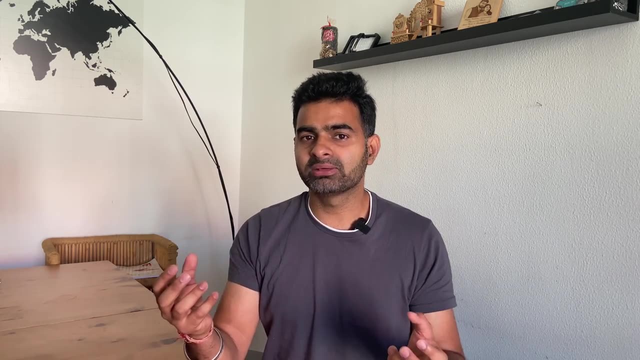 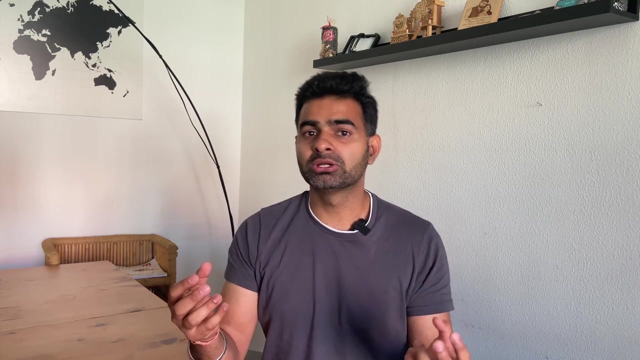 anti-replay. but that is you set right. we will discuss anti-replay and PFS in our separate video, but let's continue. in the second message, exactly same kind of information which was sent by initiator will be sent by responder. so when the first message is sent by initiator to the responder, responder will match all.